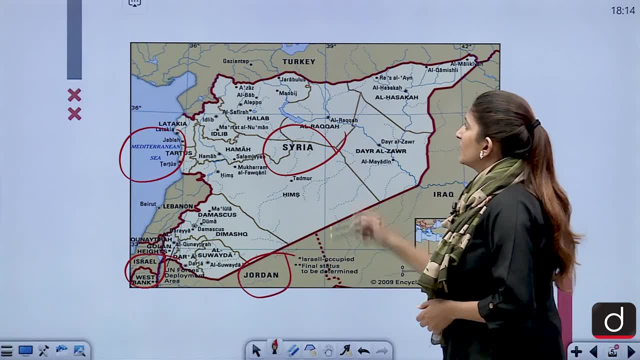 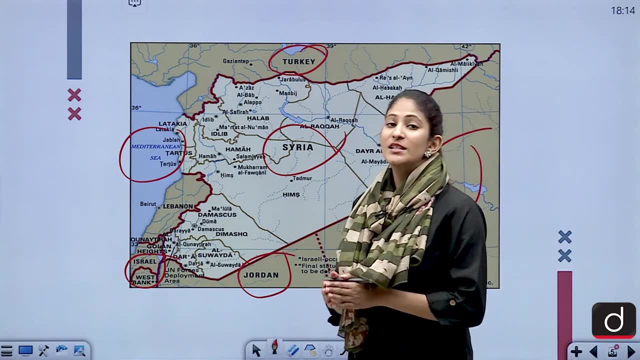 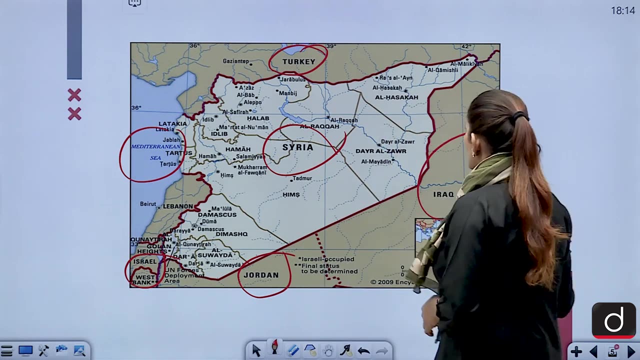 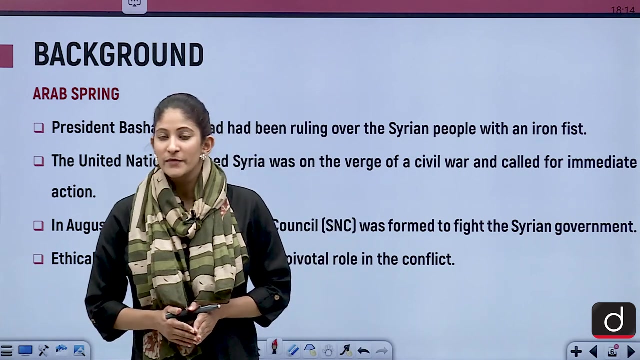 Israel, then Jordan, then Turkey. we also have Iraq, and if we talk about the largest city of Syria, you have to tell me in the comment segment and also tell me the capital of it, Alright, so if we move forward, let's talk about what has actually happened in Syria throughout that. the first: beginning of the Tekid's old war was from Arab Spring. Arab Spring actually had nothing to do with it, and even constitution making was not the demand of Syria's beginning of the war. It was actually based on when few young boys of a school drew anti-government graffitis on their school. 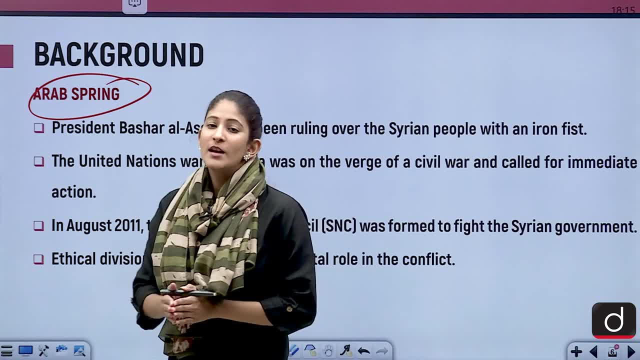 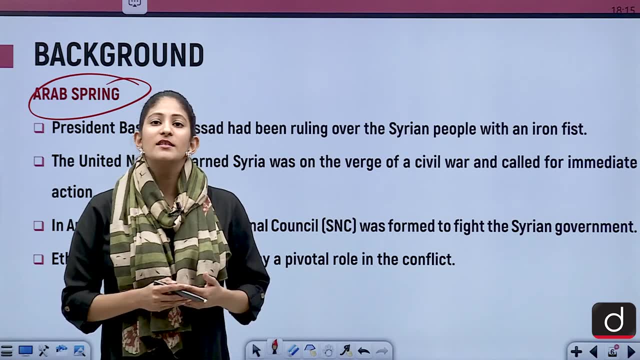 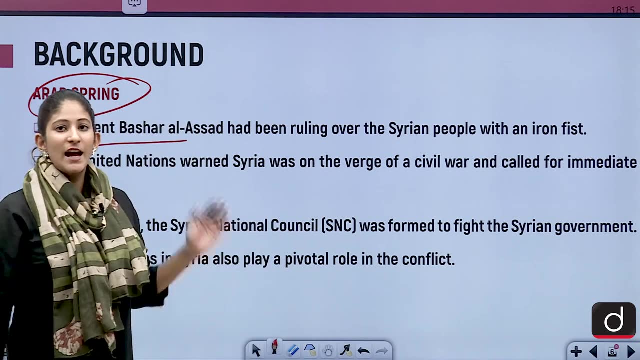 building. After that, the war, basically the clustered war and short, small scale war, started taking place and spilling over to different regions. Now, after that, President Bashar al-Assad: he had been ruling over Syrian people with an iron fist and he dealt with the Syrian people with an iron fist and he dealt with the Syrian people with an iron fist. 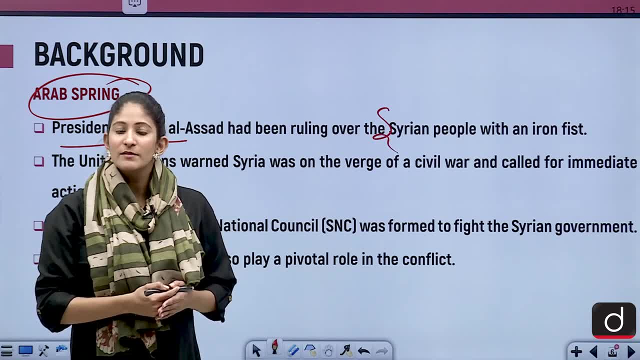 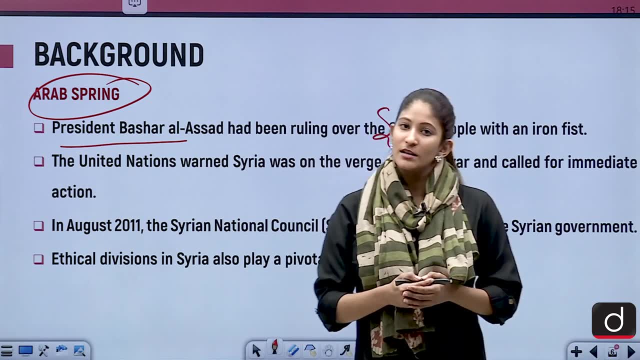 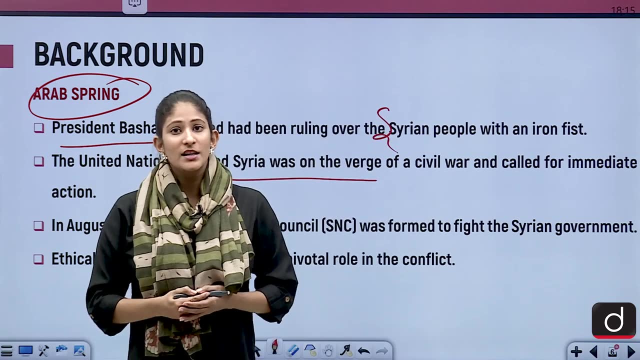 with this situation very badly after military militarizing the entire region. with this situation very badly. After militarizing the entire region, people of course understood that they wanted a reform in the governance system. After that, the United Nations did warn Syria that a civil war would take place. because of the multi-ethnicity, multi-religious structure of Syria and then, in August 2011, the Syrian national council council. it was formed to fight against the Syrian government. After that, ethical divisions started to take place in Syria and because of different ideologies. 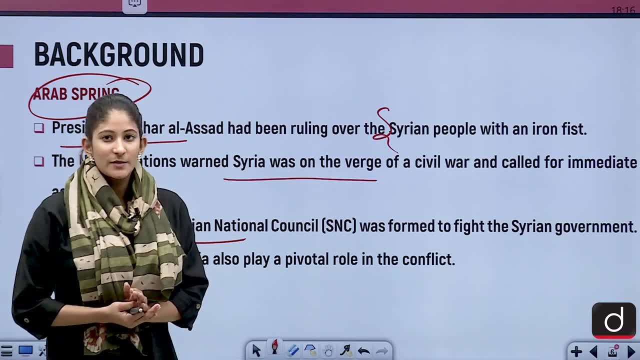 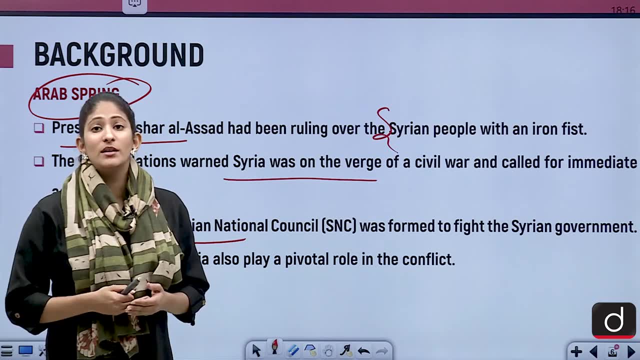 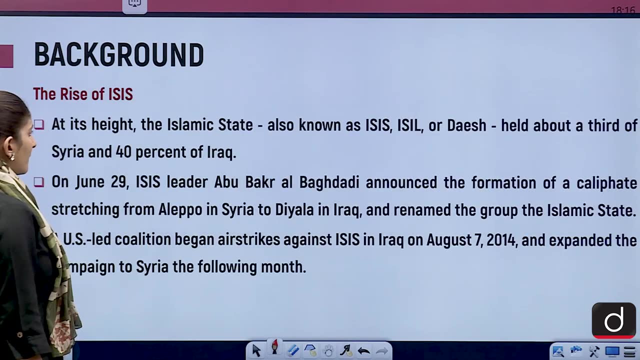 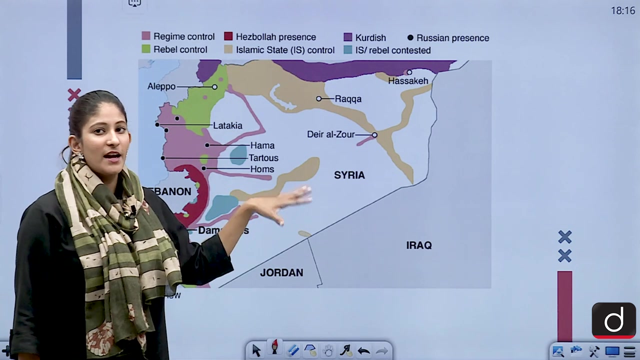 the particular sect or particular army which had been formed, and within that as well there were various ideologies, and that is why civil war started. If you could look at this map, you would come to know. Just see this map and you can understand the different colored regions were held by which? 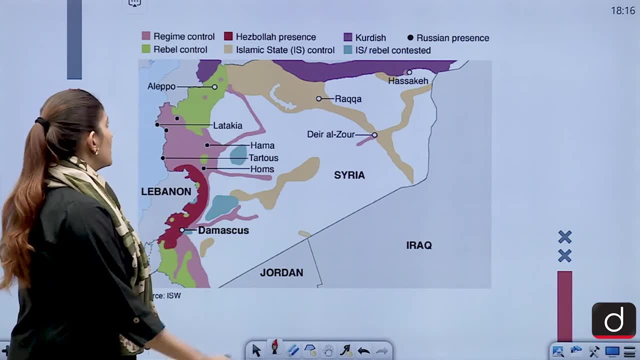 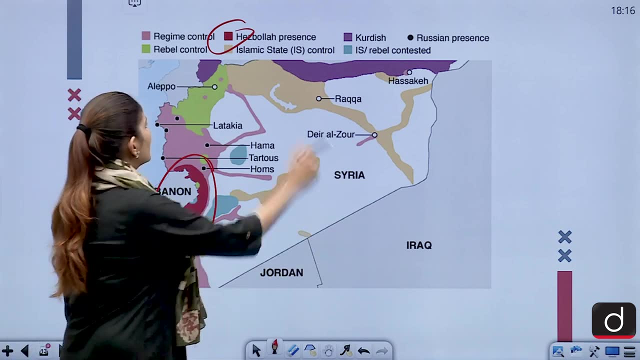 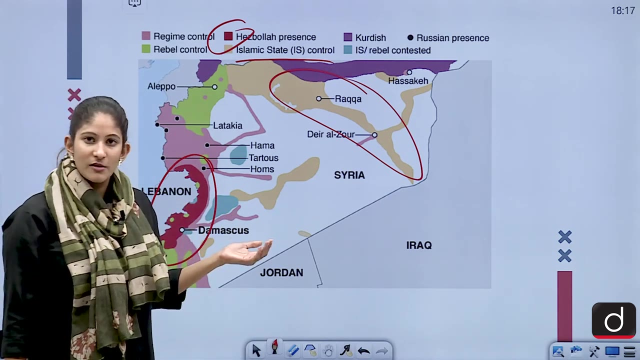 particular ethnicity, religious or ideological group. So there was Hezbollah presence over the border here right, And then comes Islamic State, of course- look at the region in yellow. then comes regime control. This is the actual, legitimate government, actual the government according to the constitution. 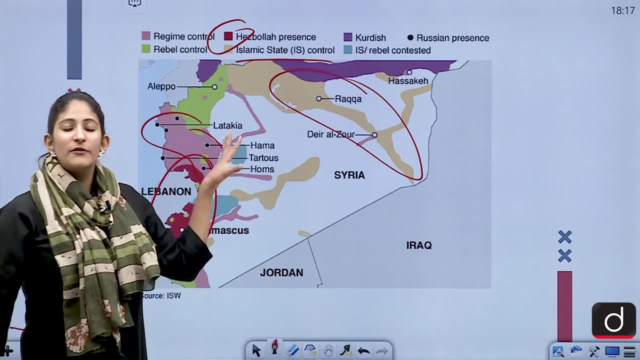 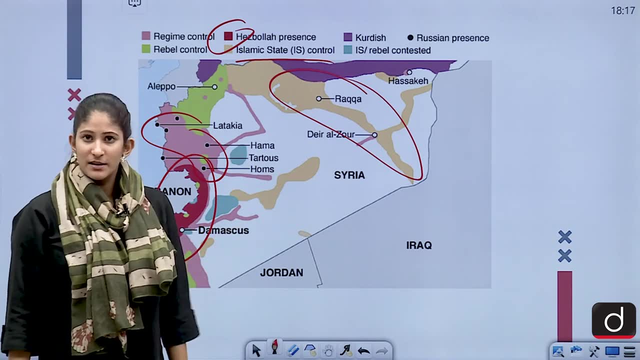 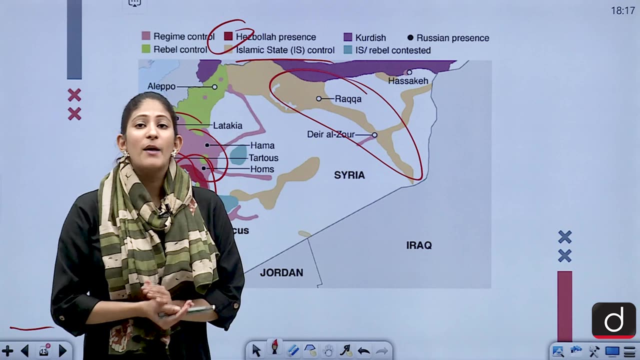 Now that's the entire pink region. So these were the different ethnicities, different religious diversities, different religious sects. They were holding control over different areas, and wherever we see difference in ideologies, religion and diversity, there is bound to be a civil war until and unless the government 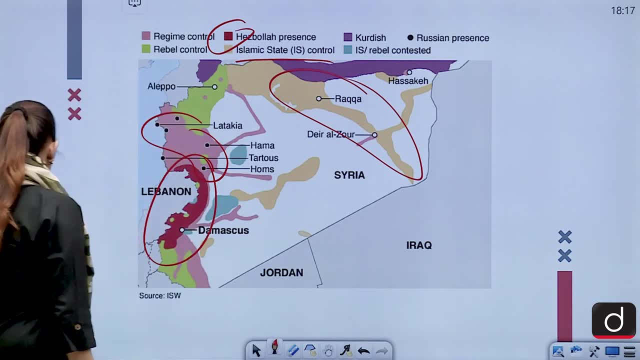 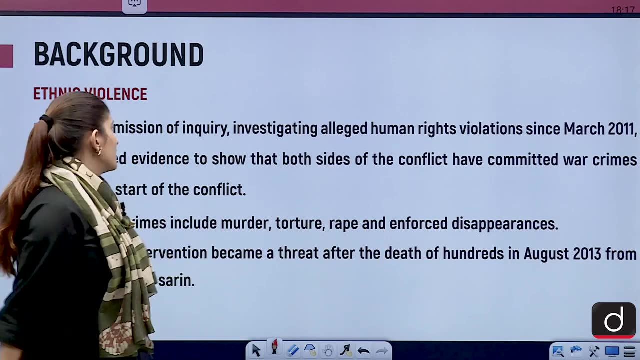 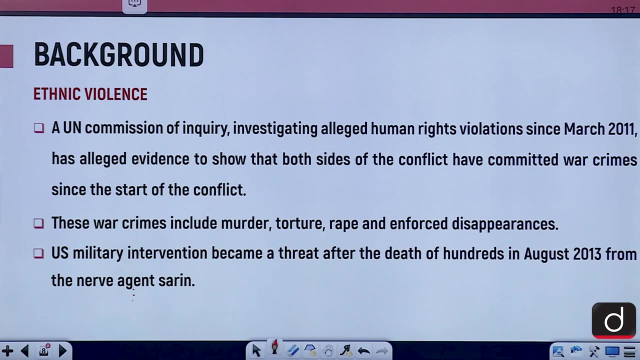 is actually democratic in nature and not totalitarian. Okay, Moving on, let's talk about ethical, ethnical violence. So a UN commission of inquiry. it started investigating alleged human rights violations since March 2011 and it has alleged evidence to show that both sides of the conflict have 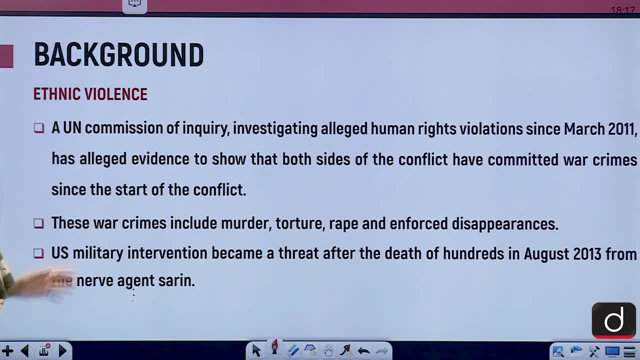 committed war crimes since the start of the conflict. Now, if we talk about the civil war, lots of murders, rapes and incitement to violence. Now, if we talk about the civil war, lots of murders, rapes and incitement to violence. 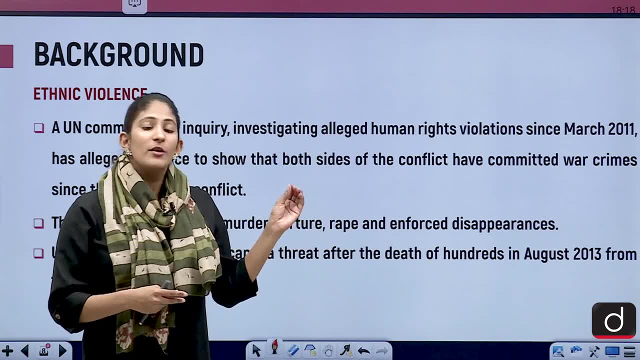 Now, if we talk about the civil war, lots of murders, rapes and incitement to violence. The civil war 오케이. so this means that we have to learn a lot about these things. A political United States. 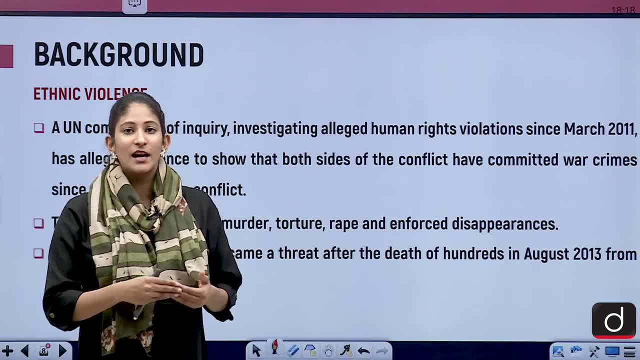 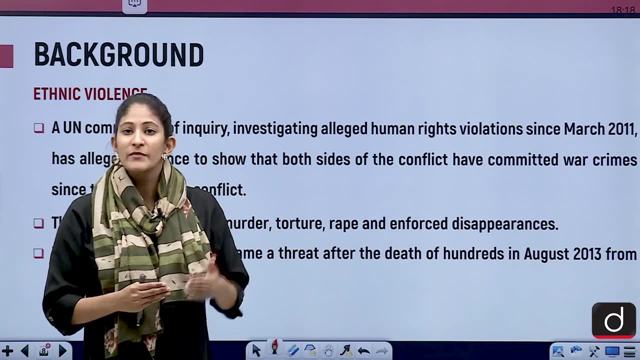 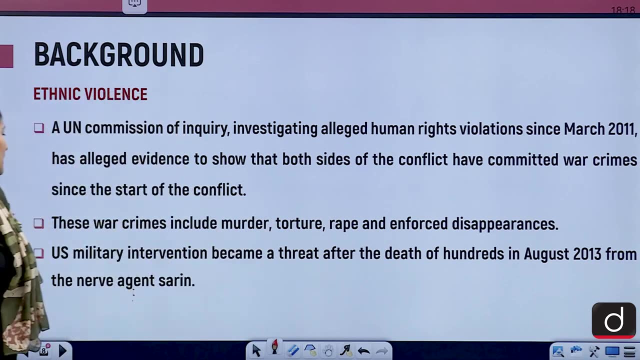 But every possible, every possible disaster and human tragedy one could imagine started happening in Syria, not only from the different sites- That means the nonlegitimate power holders and the leaders, but also the legitimate power holders, And lots of people died, and also these war crimes. of course, we told you the, including. 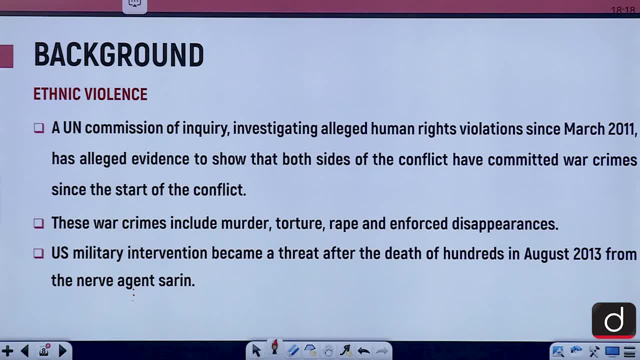 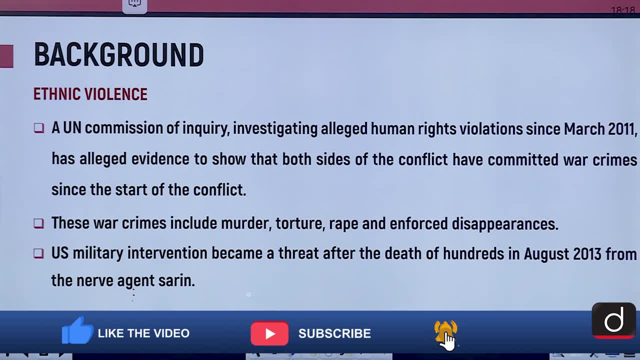 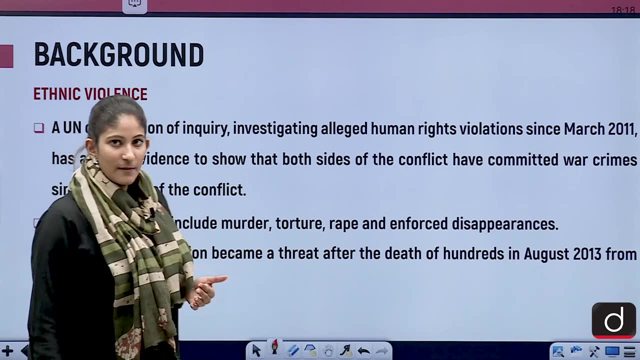 murder, torture, rape, enforced disappearances as well. Now, what happened? Whenever area or whenever a region which is actually an area of interest to the Western powers, Western powers will definitely intrude into that area. try to stabilize that region for the betterment of that region as a whole, so that it can. 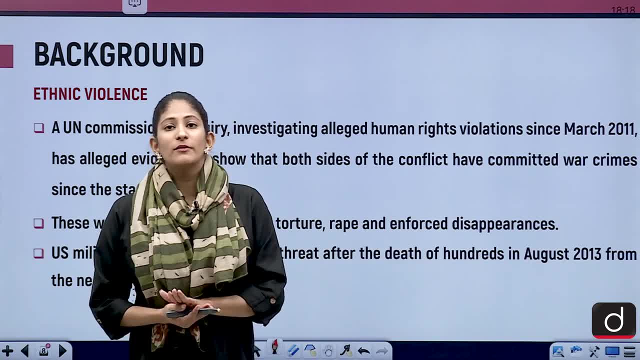 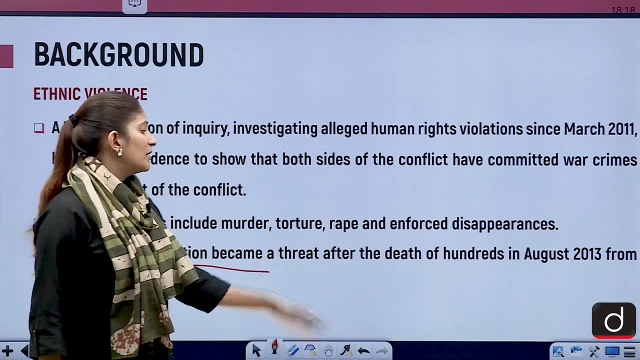 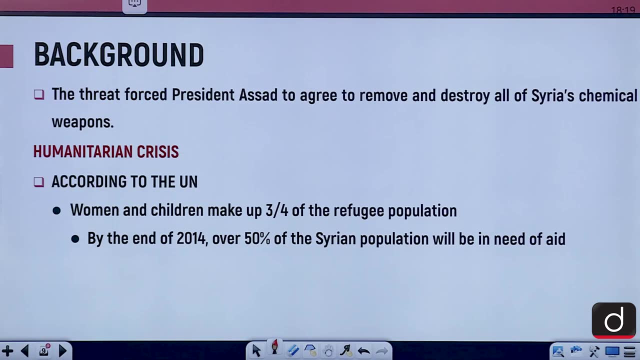 spill over and go for the betterment of the Western region. so the US military started intervening and it this intervention became a threat after the death of hundreds in August 2013 from the nerve against Saturn. now the threat forced president Assad to agree to remove and destroy all of Syria's. 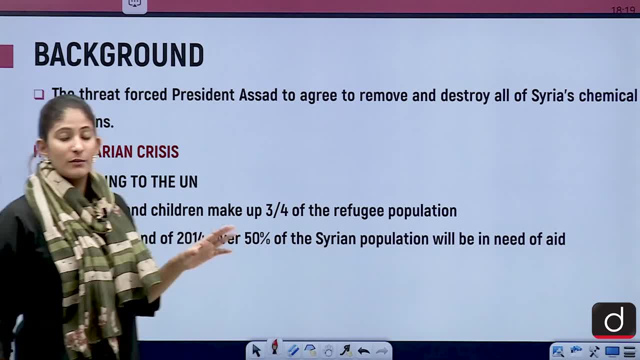 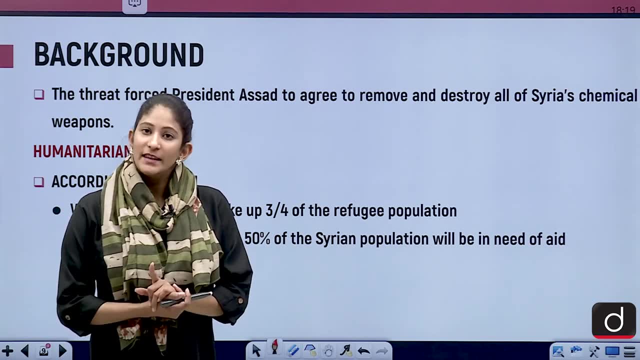 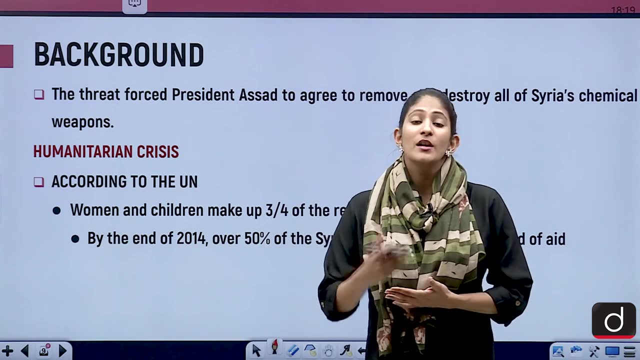 chemical weapons. so there were. the president was holding a lot of chemical weapons, which were weapons of mass destruction, and that is why this particular deed, or this particular threat which was prevailing in Syria, was stopped, was actually taken care of by the US military intervention. 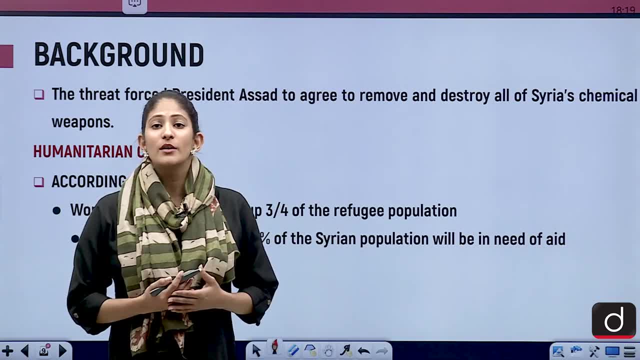 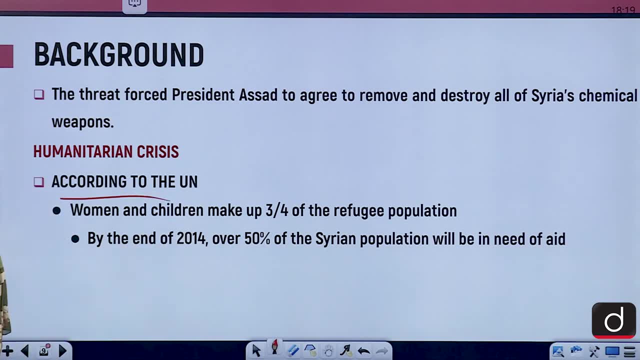 And after that we all know that it has become a playground for multi or international war right. So if we talk about humanitarian crisis, there is certain data to show it. According to the UN, women and children make up three by fourth of the refugee population. 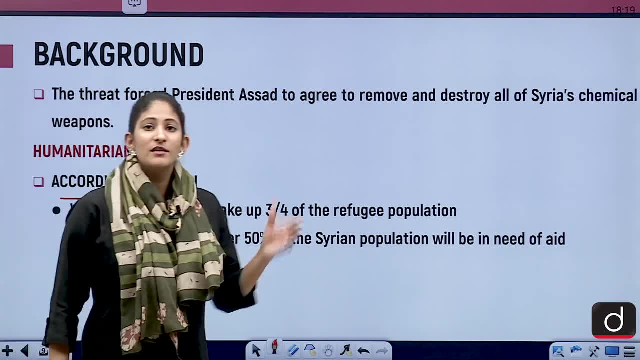 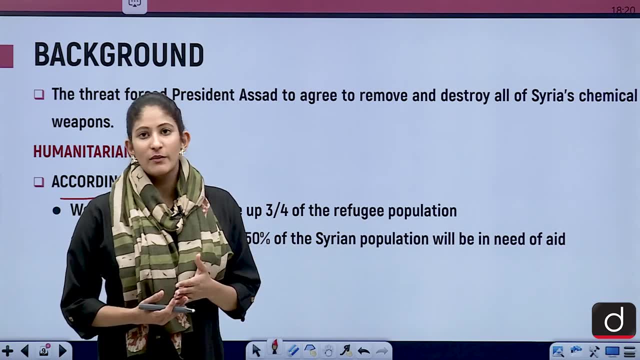 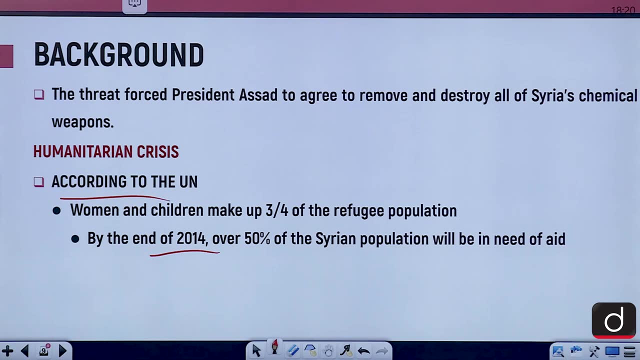 Of course, whenever a war of this scale happens, the women and the children are always at the receiving end of it, because, biologically, of course, they are the most vulnerable- Then, by the end of 2014,- if we talk about after 2000,. from 2011,, over 50% of the Syrian population will be in need of aid. 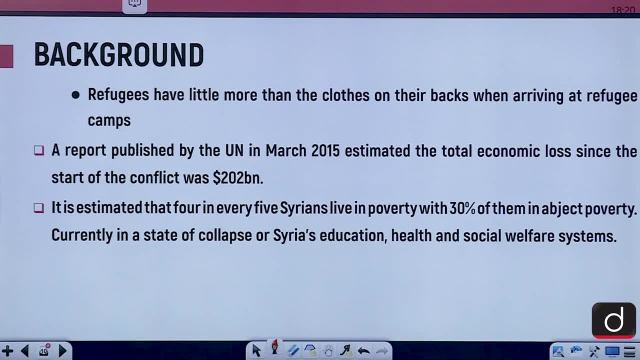 Refugees have little more than the clothes on their backs when arriving at refugee camps. A report published in the UN by the UN in March 2015 estimated the total economic loss since the start of the conflict was $202 billion. It is estimated that 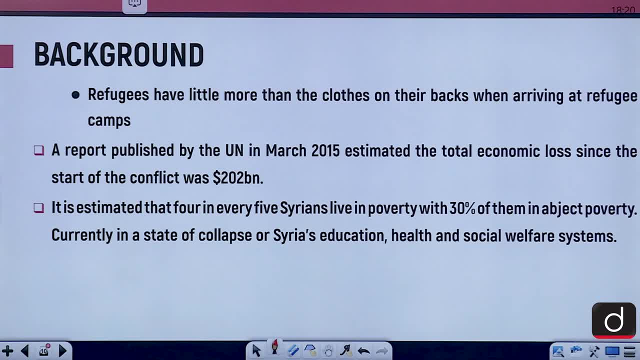 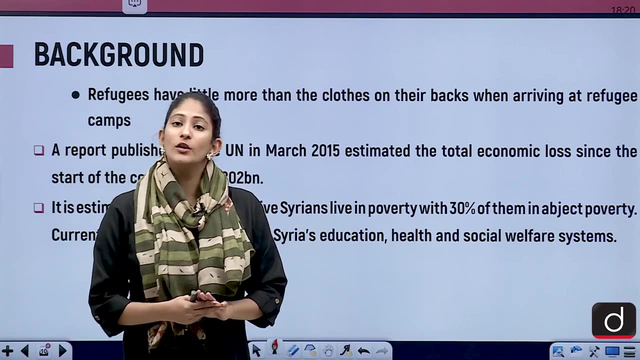 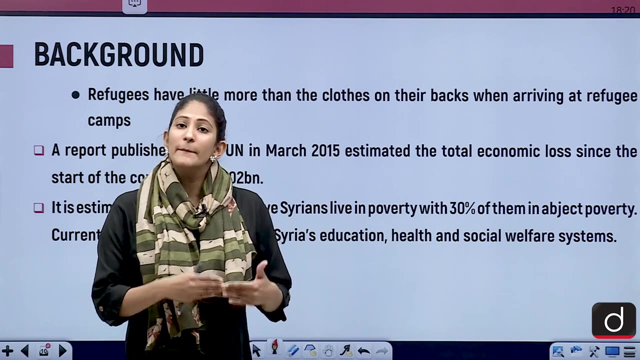 4 in every 5 Syrians lives in poverty, with 30% of them in abject poverty, currently in a state of collapse or serious education, health and social welfare system. So this region, which has been infested with war, not only sees poverty and deterioration of the entire infrastructure- social infrastructure- but also mental health. 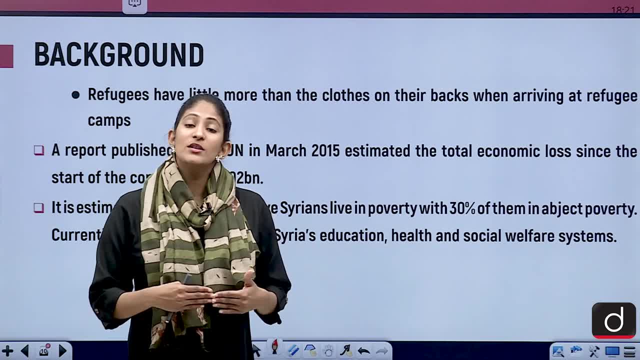 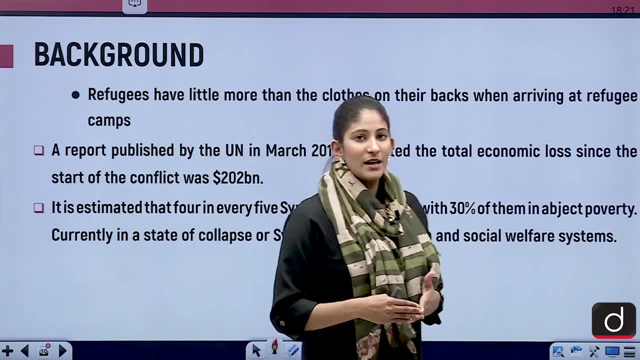 It is taking a toll on the mental health of the people. They have no hopes for the future. The war has been so prolonged And now again the new constitution which is to be made. it's taking a lot of time And US and its western allies are accusing the president. 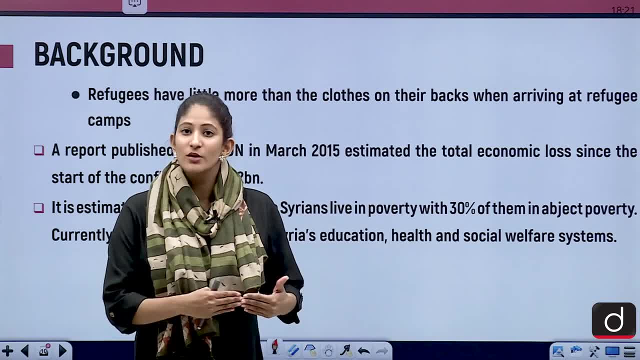 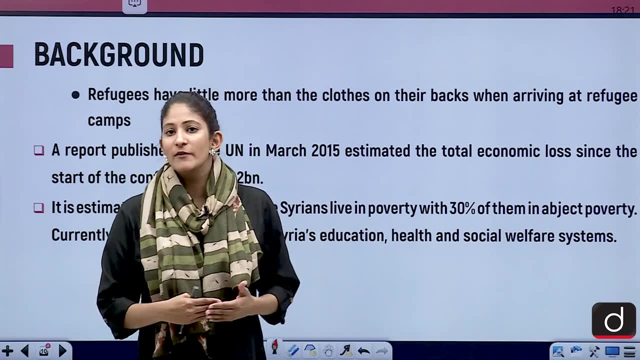 President? why? Because they are saying that he is trying to delay the election. He is trying to delay the constitution making process so that the election arrives and he can have his own way there. Moving on, let's talk about the rise of ISIS. 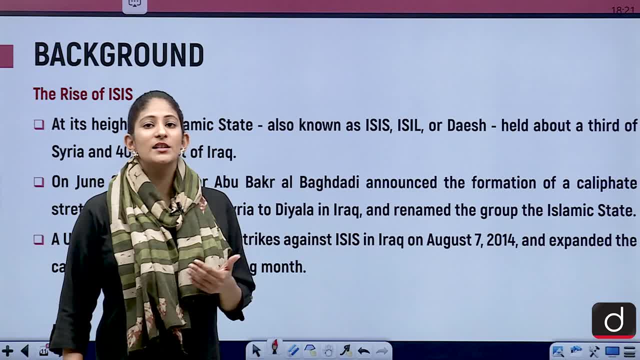 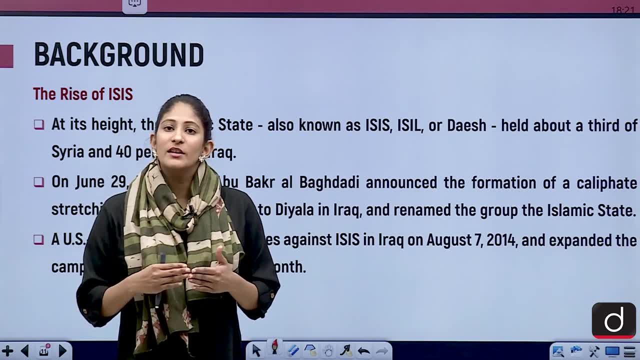 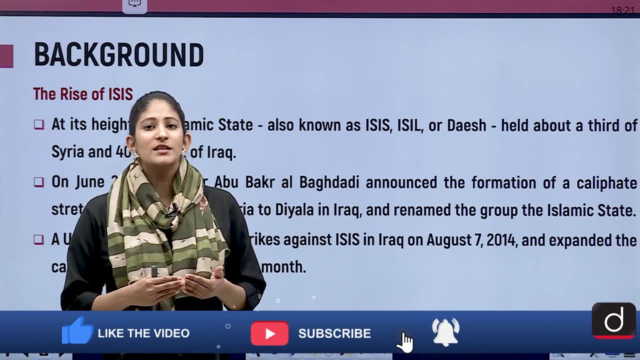 So There was a political vacuum. The political structure was in a dilapidated state, And whenever there is a lack of proper ideology or there is a lack of proper or coordinated coordination between the government machinery and the diversities living there, the vacuum will always be filled negatively. 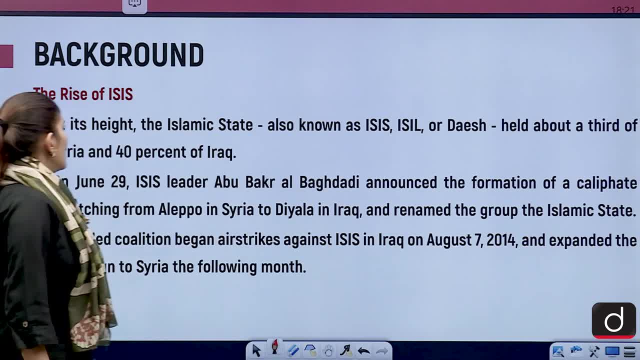 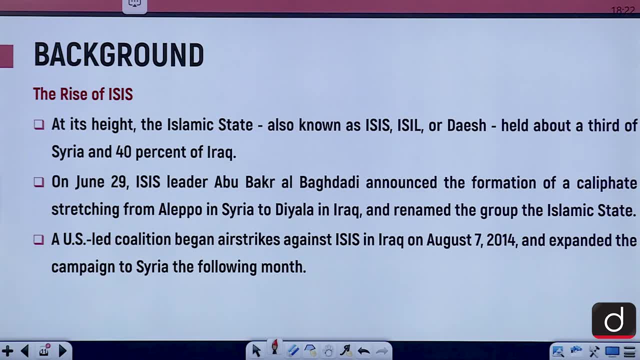 Here what happened. ISIS emerged. So, at its height, the Islamic State, which is also known as ISIS, ISIL or Daesh, held about a third of Syria and 40% of Iraq On June 29,. ISIS leader Abu Bakr al-Baghdadi. this was in 2015,, by the way. 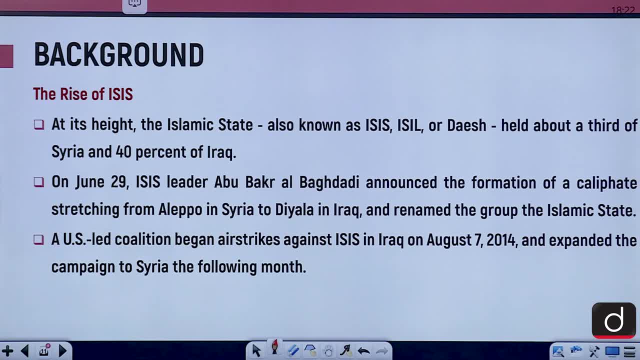 he announced the formation of a caliphate stretching from Aleppo in Syria to Diyala in Iraq and renamed the group the Islamic State. Now, the US-led coalition began airstrikes against ISIS in Iraq on August 7, 2015.. And expanded the campaign to Syria the following month. 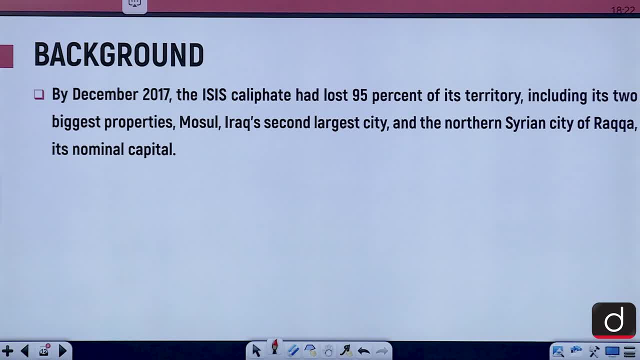 By December 2017,, the ISIS caliphate had lost 97% of its territory, including its two biggest properties: Mosul, which is Iraq's second largest city, and the northern Syrian city of Raqqa that is its nominal capital. 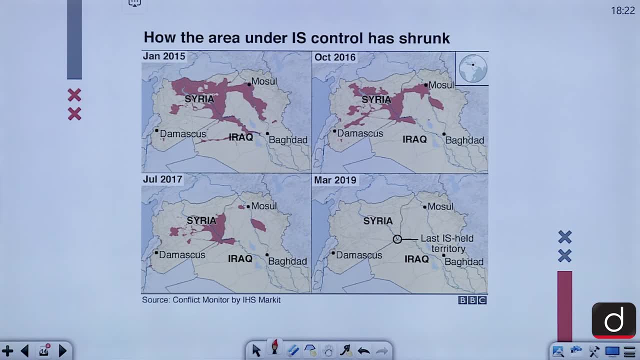 So if we look at this particular map, see in January 2015, it was ruling over so much quantity of land. So if we look at this particular map, see in January 2015, it was ruling over so much quantity of land. 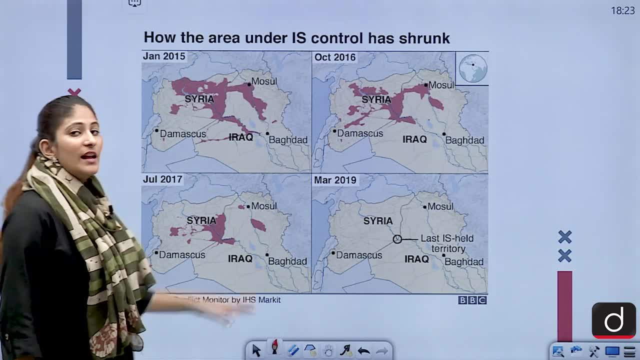 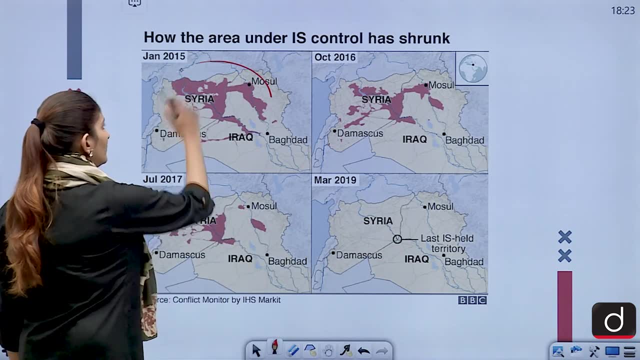 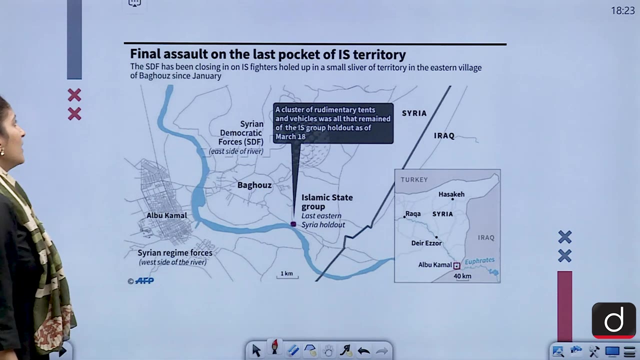 And now, if we talk about March 2019, it has lost most of its rulings over the lands in that particular region. So this was because of international intervention And if we talk about this news, it shows that final assault on the last pocket of IS territory. see. 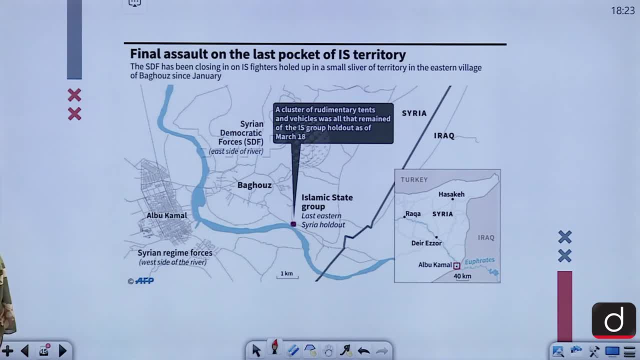 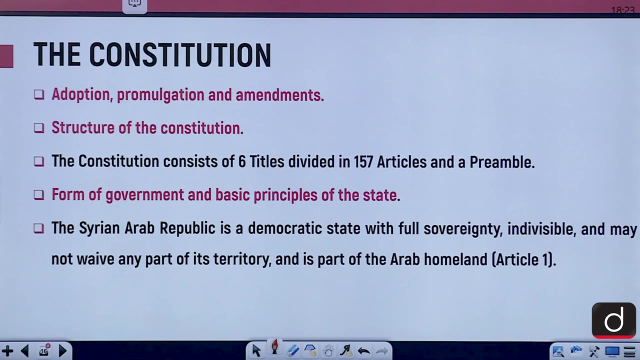 a cluster of regimentary tents and vehicles was all that remained of the IS group holders, And this is from 2019.. So, moving on, If we talk about the constitution, the constitution making process which started since there was a constitution in 1973. 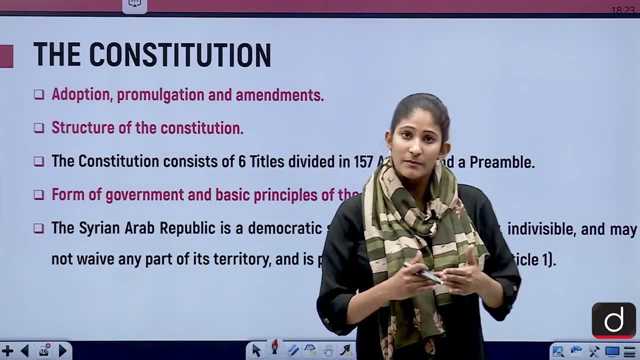 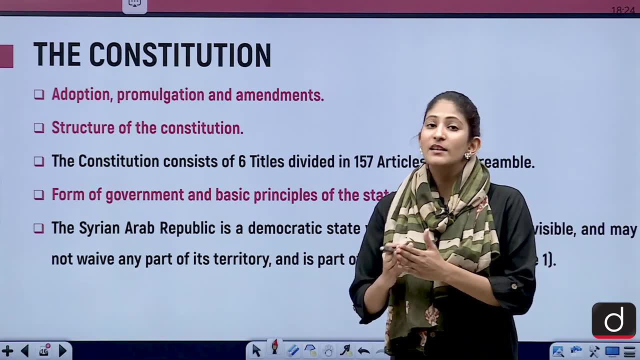 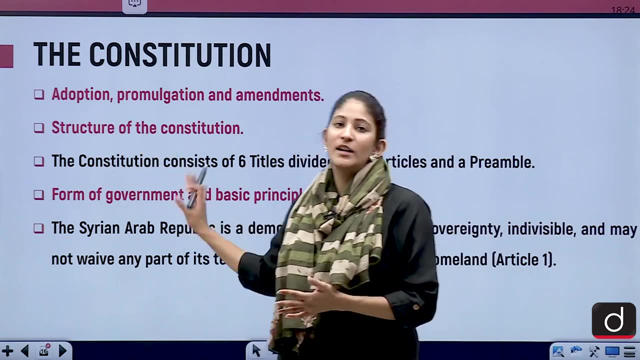 And that particular constitution said that the Baathist party was the head of the state and the society, And that particular article, article 8.. It showed that, yes, Baathist party was the society's and particular, it was the head of the entire country that it was wanting to say. 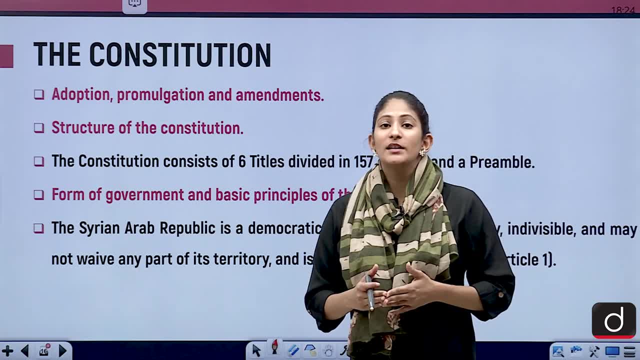 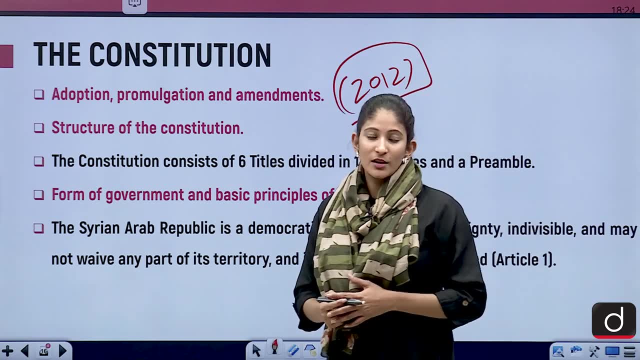 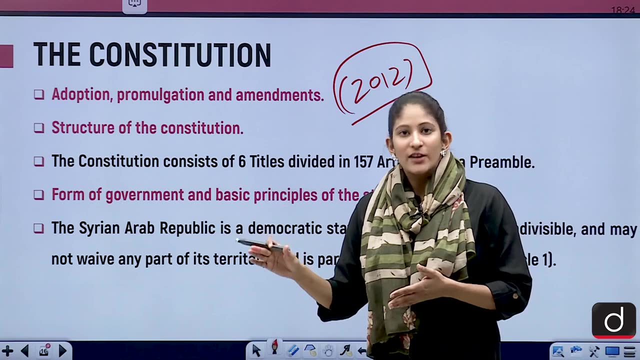 So the people did not want that. After that, in 2012,, there was a call for reformation in the constitution And after that, the president he elected without any election. He nominated few members Of the Baathist party, non-Baathist party and many other groups as well. 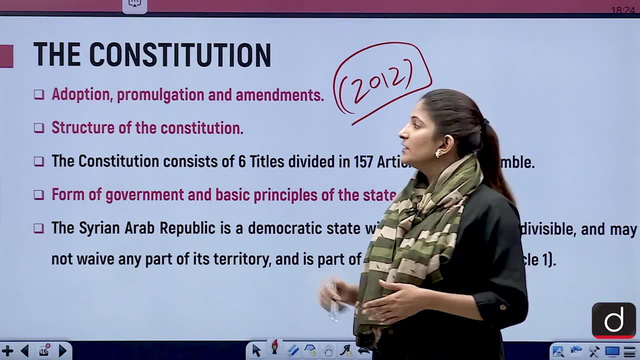 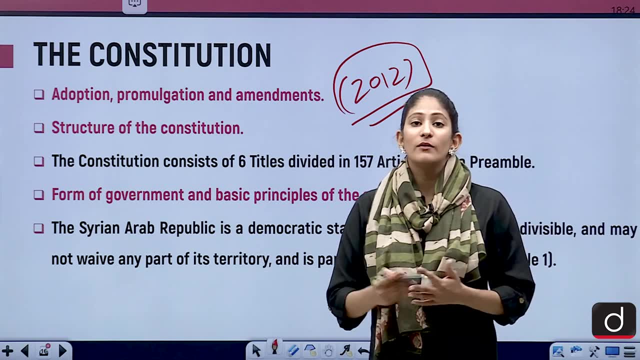 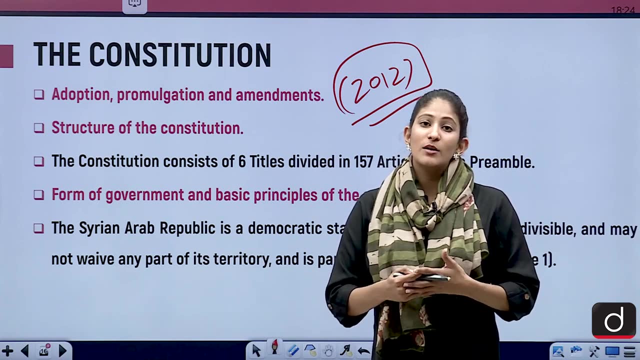 But they were non-elected in nature, And that is why the 2012 constitution which was formed was outrightly rejected by many of the groups By saying that this does not show the democratic mindset of the government, Because it is not this constituent assembly which has drafted the constitution of 2012.. 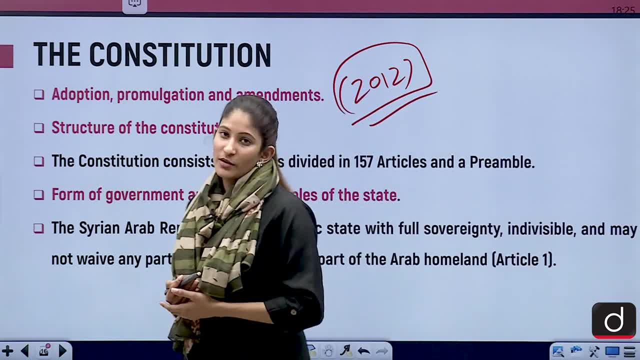 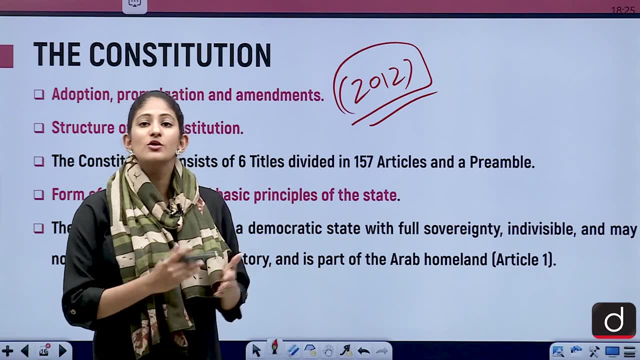 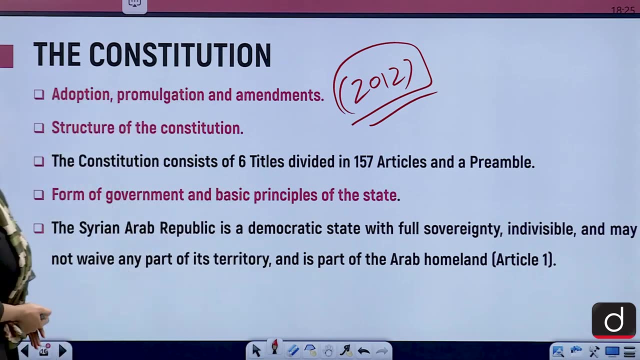 That is non-democratic, It is not democratic in nature, It is undemocratic. So that is why this particular constitution needs a reform, Because this constitution shows nothing but the president's totalitarian state of mind- Not democratic. So if we talk about the structure of the constitution, 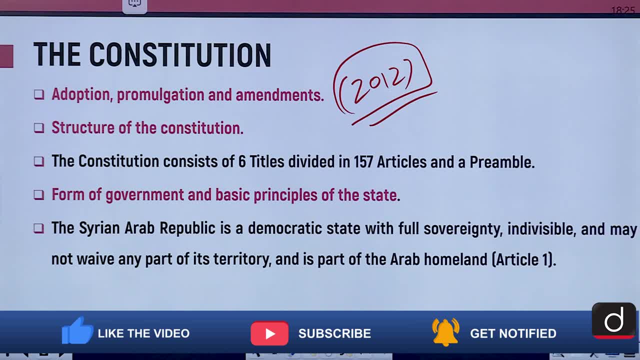 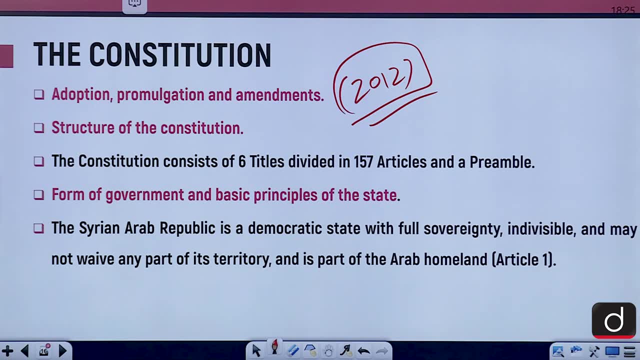 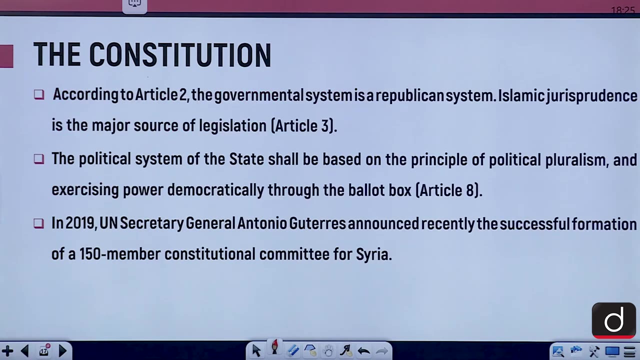 The constitution consists of six titles divided in 157 articles, and there is also a preamble, If we talk about the form of government and basic principles of the state. The Syrian Arab Republic is a democratic state with full sovereignty, indivisible and may not waive any part of its territory, and is a part of the Arab homeland according to article 1.. 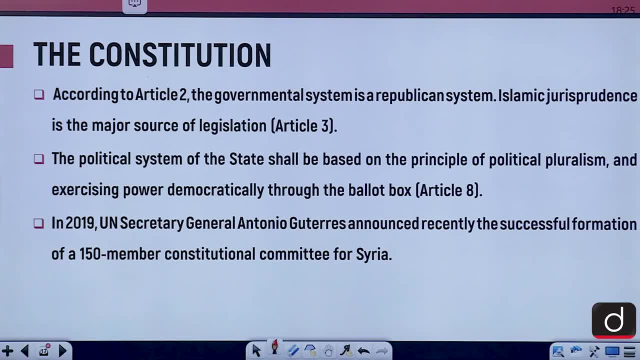 According to article 2,, the governmental system is a republican system. Islamic jurisprudence is the major source of legislation. The political system of the state shall be based on the principle of political pluralism And exercising Power democratically through the ballot box. 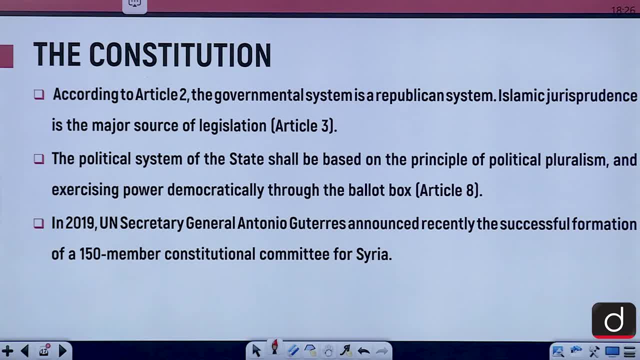 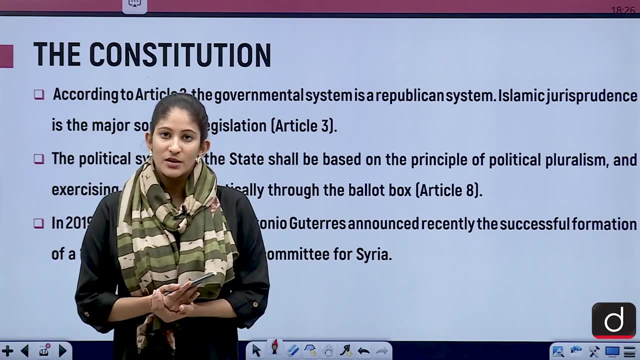 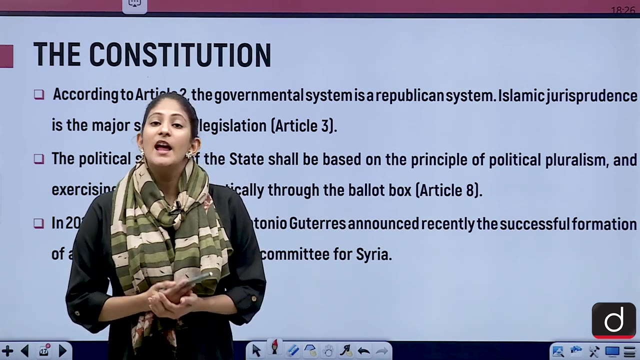 In 2019, 18-19 basically. UN Secretary General Antonio Guterres announced recently the successful formation of a 150 member constitutional committee for Syria And when this committee was formed, when this committee was formulated, it was supported by the five members, five permanent members of the United Nations Security Council and many other countries. 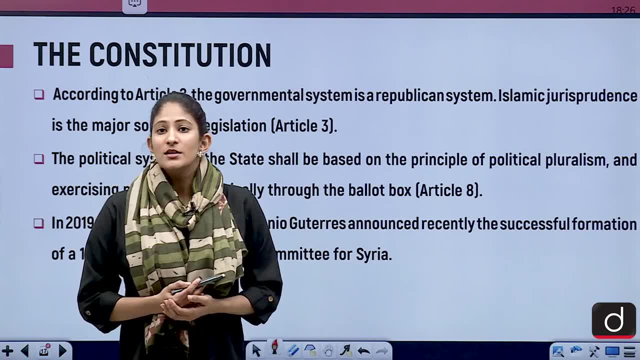 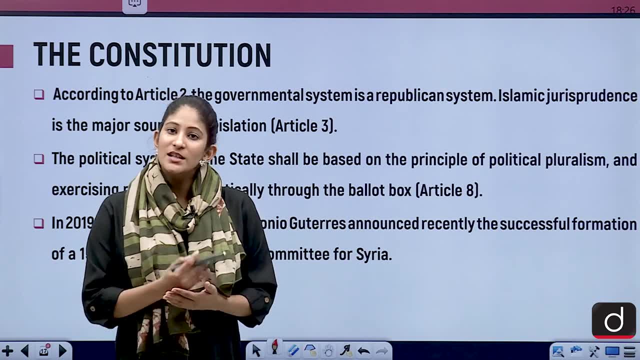 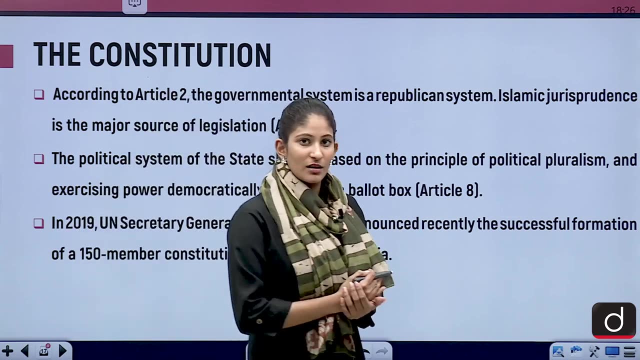 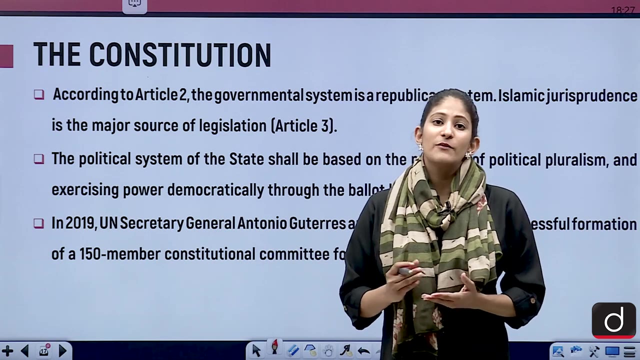 Which are big, There is a big world. So, if we talk about the legitimacy of this constituent assembly, it is backed by the United Nations. and what does it want to do since the year 2012,? it is trying to make reformation in the constitution and the structure- political structure- of Syria so that the peaceful coexistence between different ethnicities and religious groups exist right. 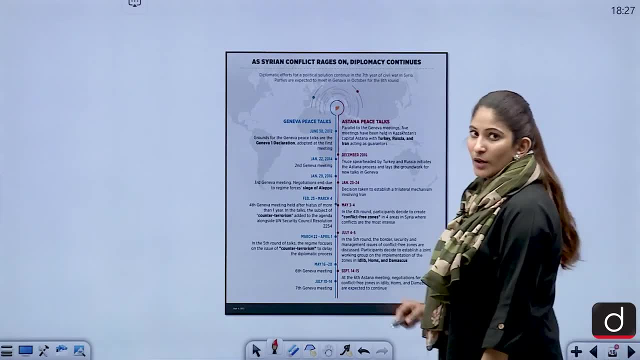 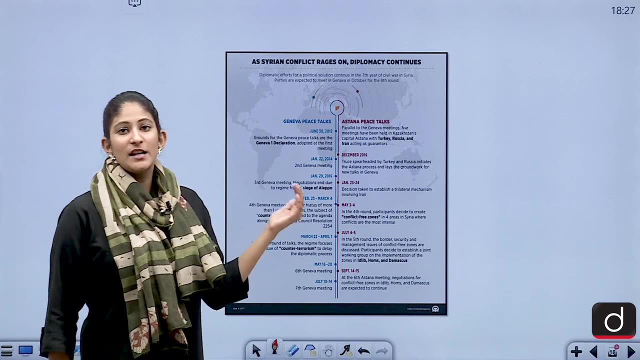 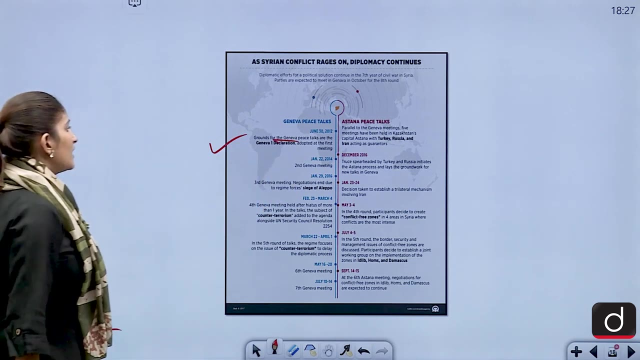 So that it is what is one want to Do. It wants to do that only. So if we talk about 2012,, then begins the Geneva communique and it says: grounds for the Geneva peace talks are the Geneva one declaration adopted at the first meeting, and after that rounds of different Geneva meetings was happening. 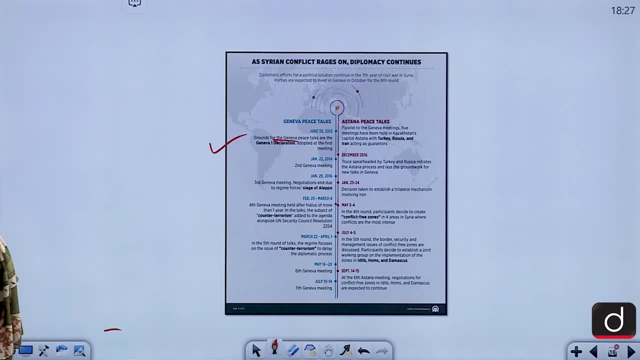 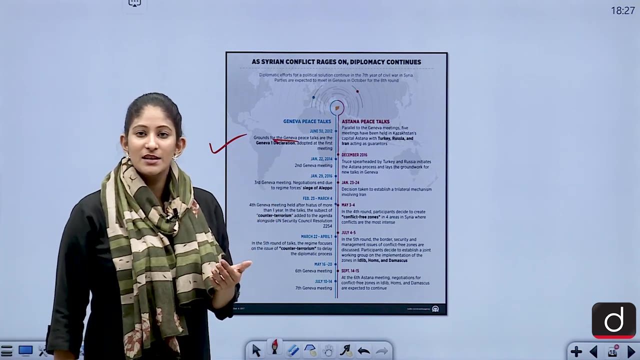 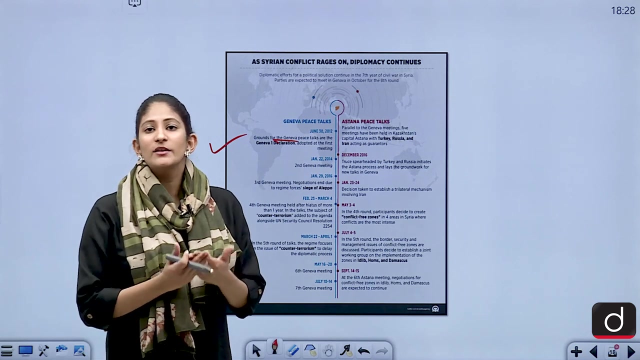 Now the third Geneva meeting was happening and then then negotiations Ended Due to regime forces siege of Aleppo and after that, because of the rise of ISIS. now what happened? United Nations had this role of peaceful transition of the war-torn country, but what happened? because of the rise of the ISIS? then came making of the constitution and also fighting terrorism. 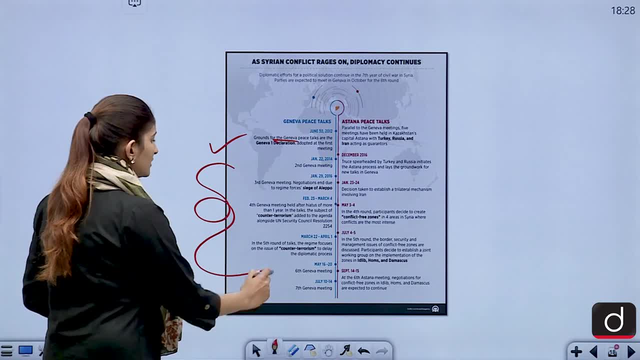 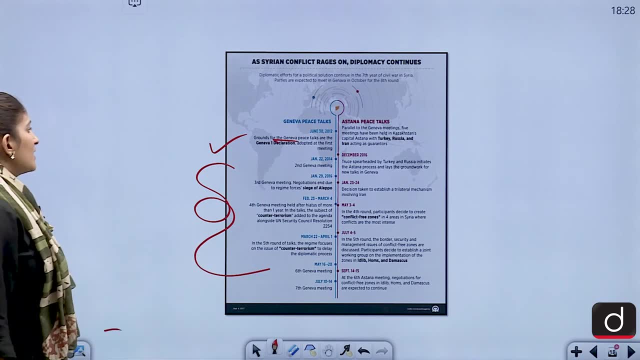 So these particular counter-terrorism strategies had to be held alongside, So these particular counter-terrorism strategies had to be held alongside, So these particular counter-terrorism strategies had to be held alongside The constitution making process. after that, when Astana peace talks began, they began parallel to the Geneva meetings. five meetings have been held in Kazakhstan capital, Astana, with Turkey, Russia and Iran acting as guarantors. 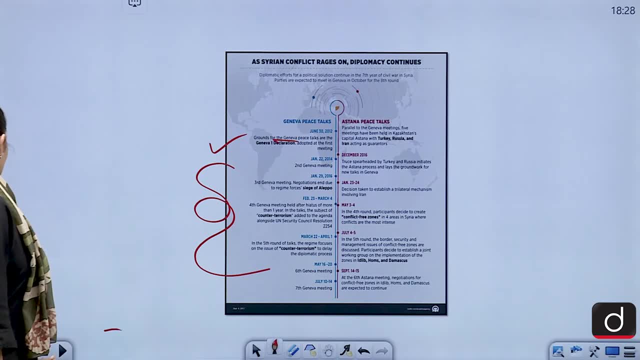 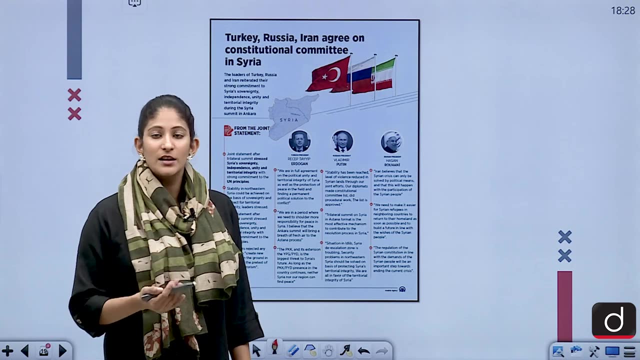 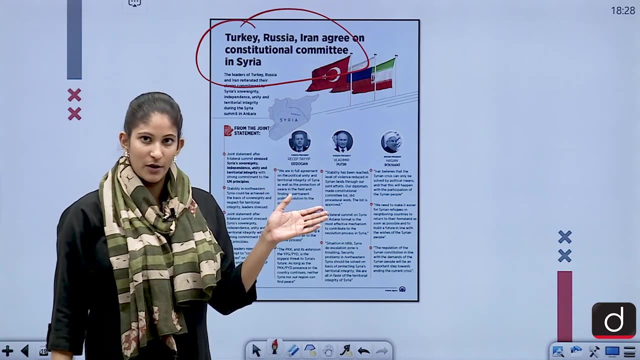 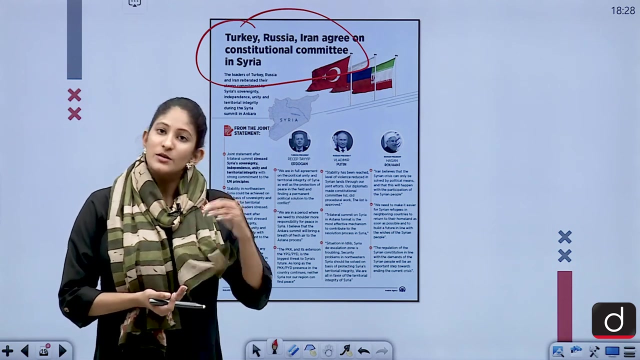 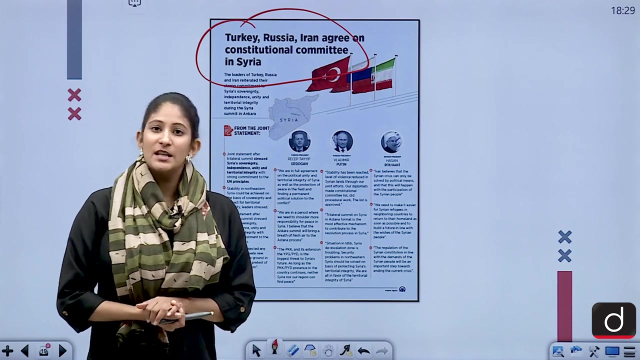 And also if we talk about the guarantors, the guarantors if we talk about the important countries which have stakes there: Turkey, Iraq and Russia, Turkey, Iraq and Russia. They all agreed on the formation of the constitution committee for Syria because these countries, in order to be economically stable, in order to be socially, socially, in the sense, geopolitically- stable, they need Western region, Western Asia, to be stabilized. 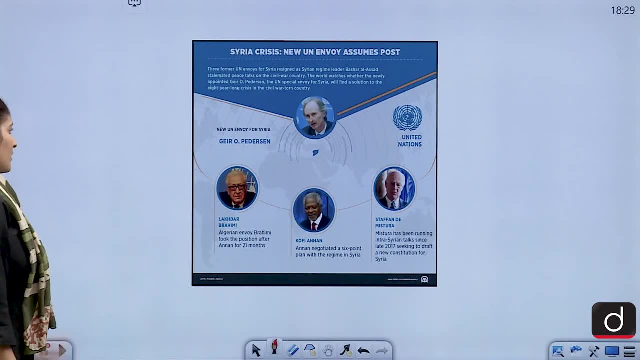 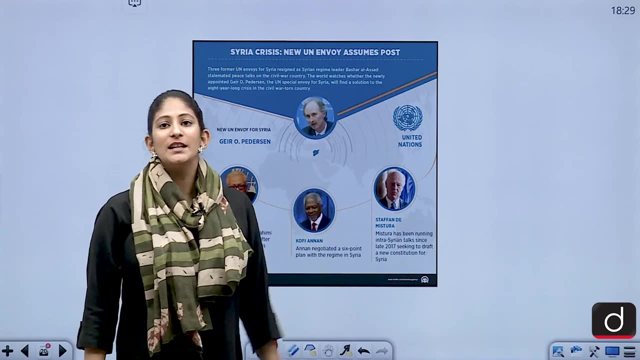 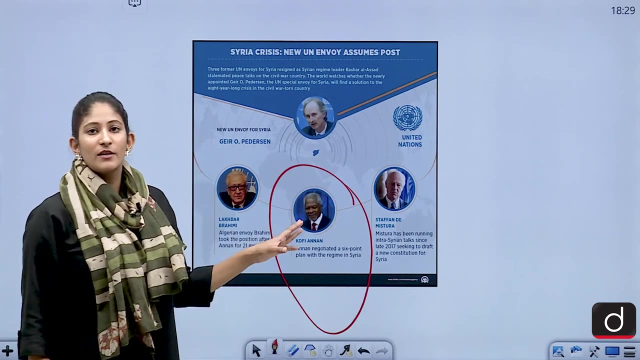 So they had their own reasons for the stability of Syria. and if we talk about UN United Nations, So they had their own reasons for the stability of Syria. and if we talk about UN United Nations, Now the first ever step that was taken by person from the UN, it was by late Kofi Annan. 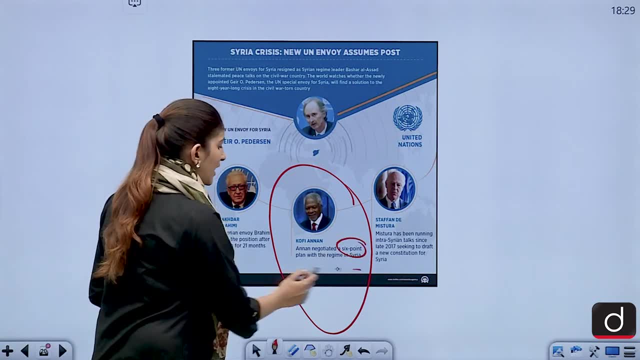 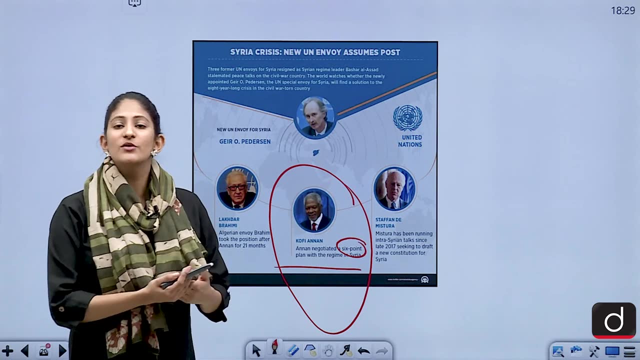 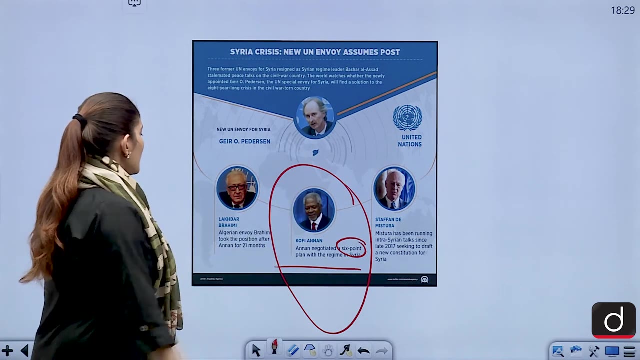 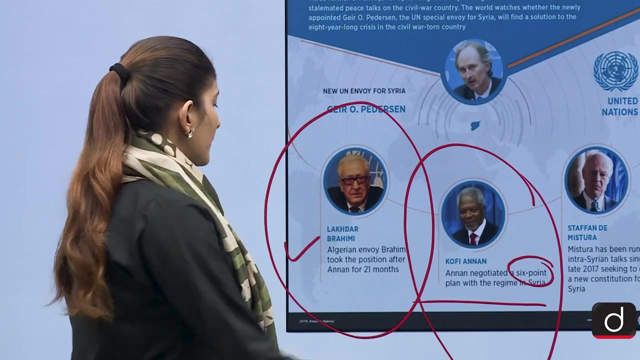 Now he negotiated a six-point plan with regime in Syria, and constitution making was not a part of it. There was just peaceful transition from the war-torn country to a stable, democratic country. After that, Lakhdar- Now he was an Algerian envoy to take the position for 21 months after Kofi Annan. 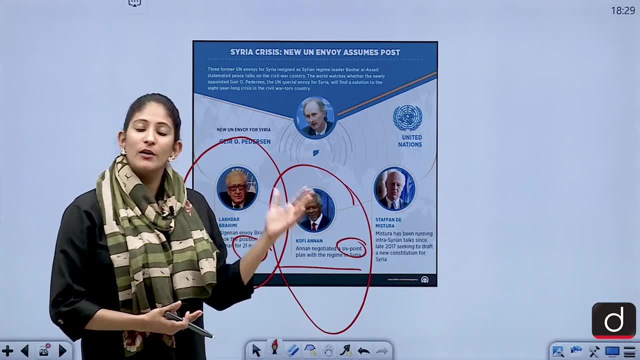 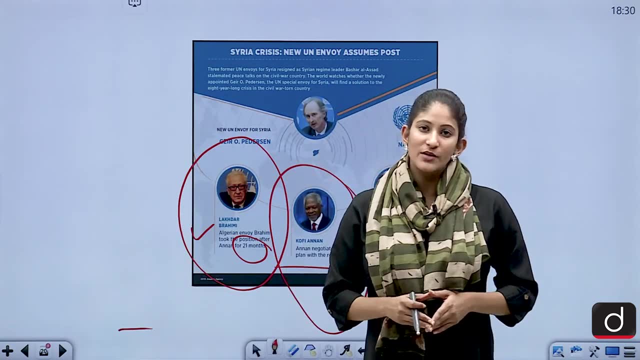 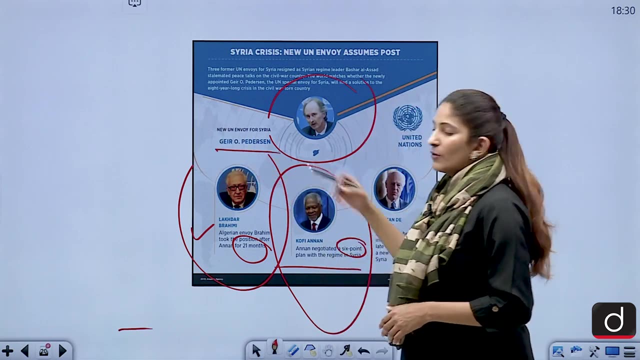 Now all these director generals, all these people. they were trying to not bring a constitution into being but, of course, peaceful transition After that. now, the new envoy by the name of Gero Pedersen. He says a constitutional reform is needed. 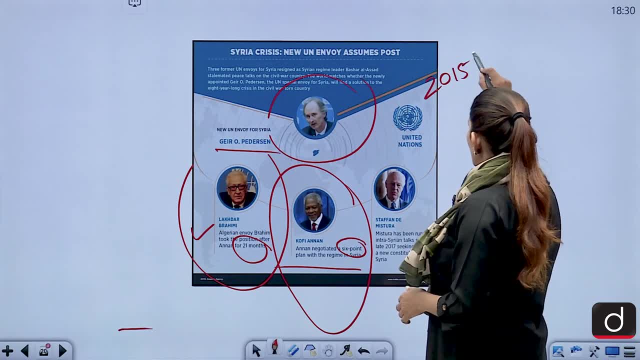 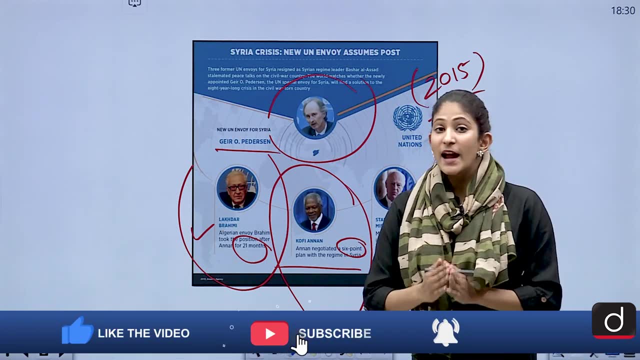 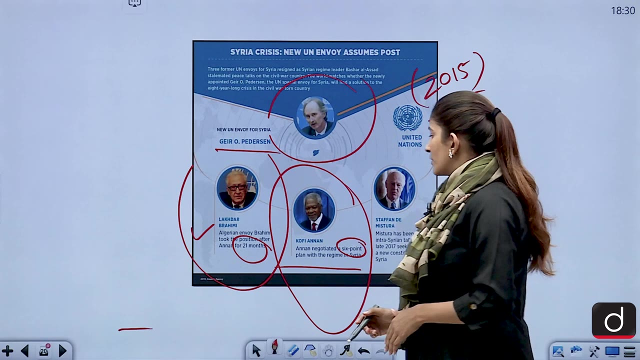 So in the year 2015, A United Nations, United Nations resolution was passed and after that, the constitutional seats were grown That, yes, we do need the drafting of a new constitution. So this, as you can see, was built step-by-step Right. 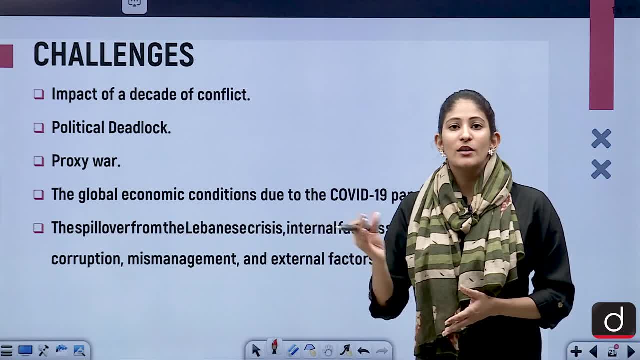 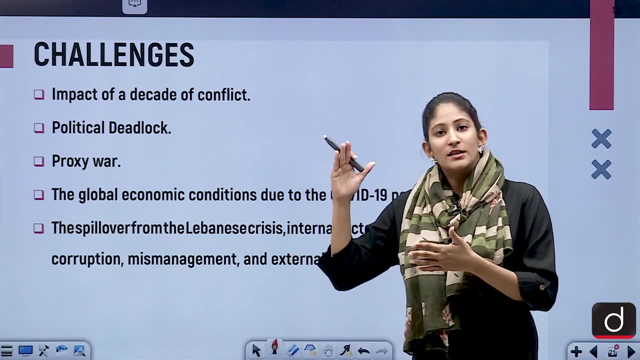 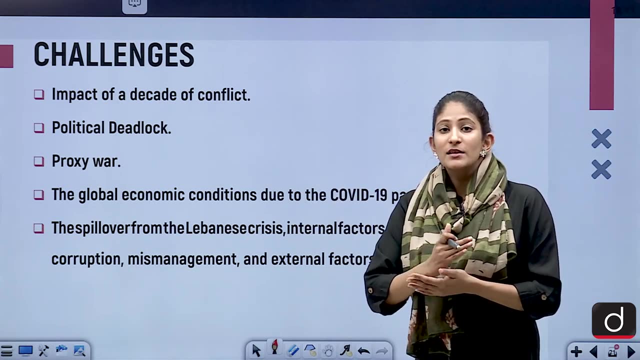 It wasn't from the very beginning. Yes, constitution, a constitution should be made and a constitution should be intervened with the help of the UN. They never, the United Nations never said that they wanted a constitution from the beginning. But after they saw what the actual problem there is, where the actual problem lies, they 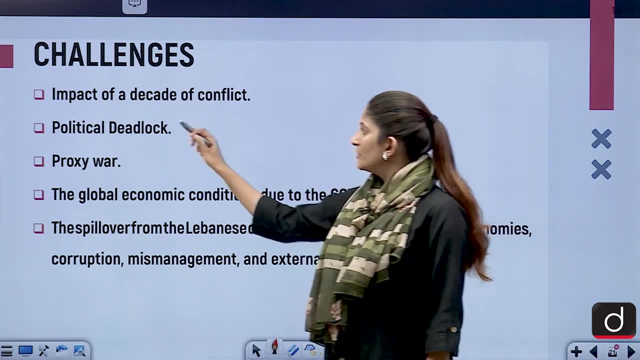 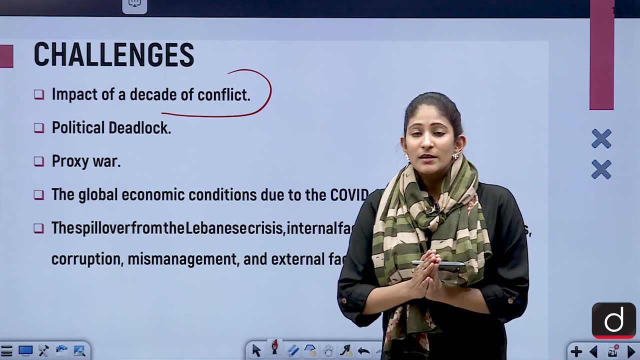 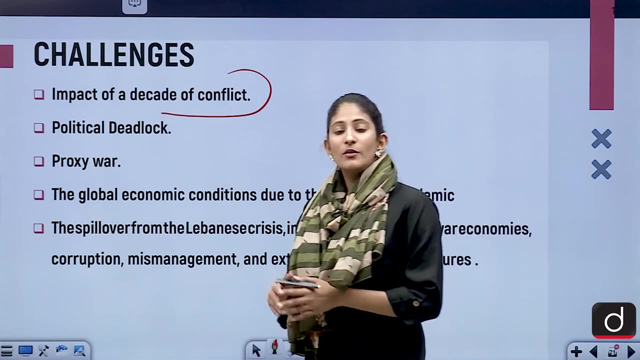 started with their constitution making process. So, if we talk about the challenges, first challenge now is that their country, Syria, has been warnt on since more than a decade now. Now, if we talk about the status of the country, the status of the country is such that it 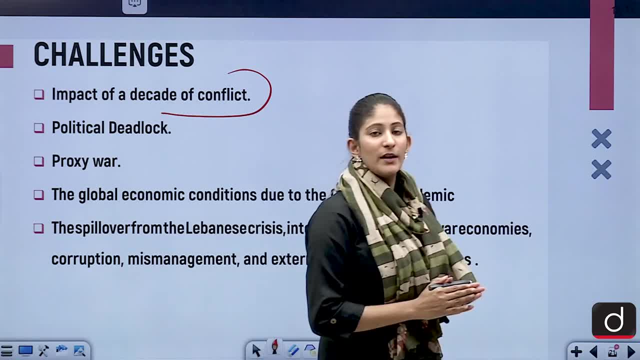 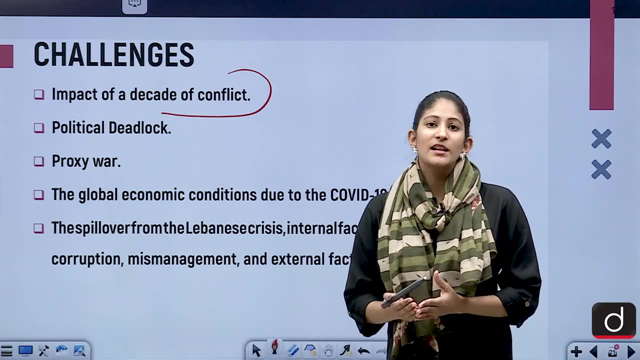 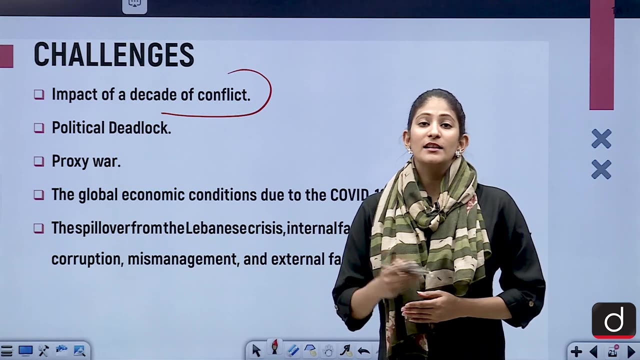 has no proper system when it comes to the political structure, when it comes to the human resource structure, When it comes to the basic infrastructure. the psychology of the people there has been divided because so many ethnical as well as religious diversities exist. 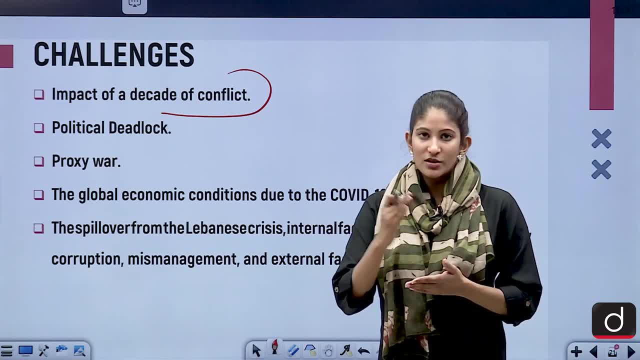 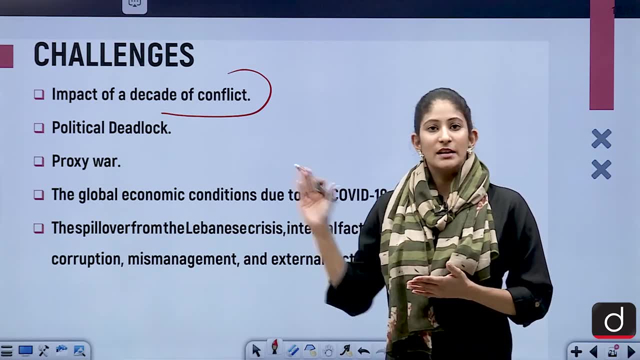 So the biggest challenge here is first to restructure the entire country. when it comes to political, economic, social, environmental- you name it, they have it. So the first challenge is that political deadlock. So many ethnical diversity, So many religious. 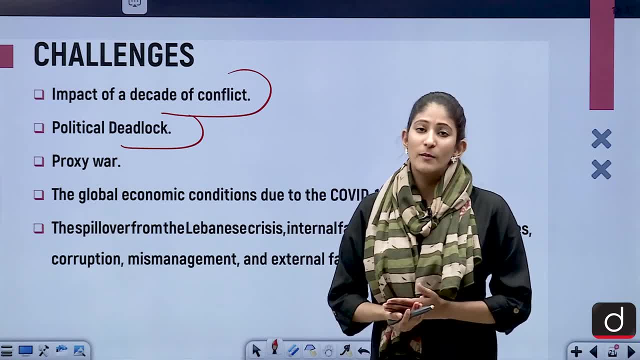 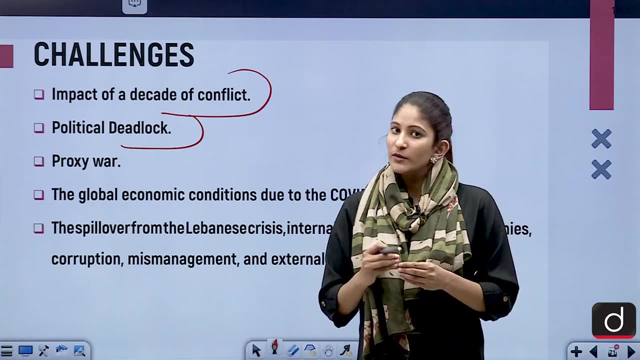 So many religious diversity, So many ideologies, So many groups have been formed. The political deadlock there exists. So bringing them at one table without the help of the military is the second challenge. Proxy wars: Now so many countries are involved. 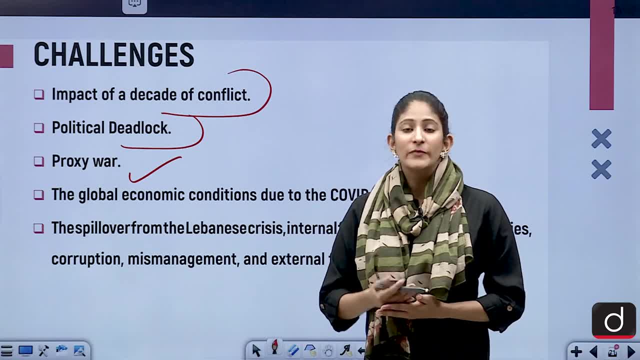 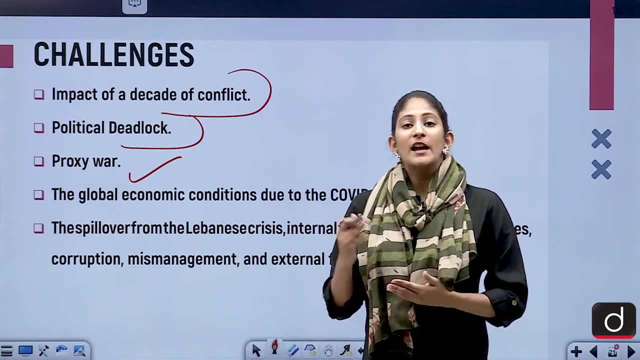 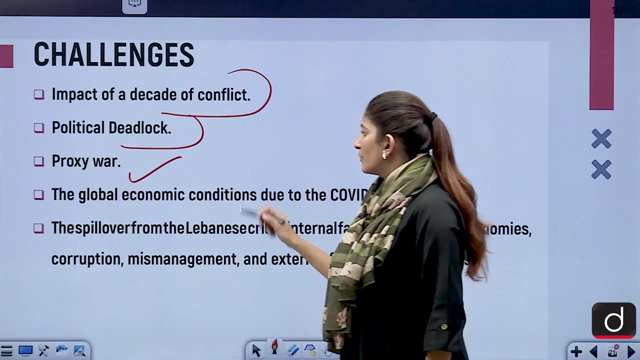 The involvement of US, Russia, Iraq, Turkey. so many big players are there in this particular region that everybody is fighting for their own, Their own betterment or their own reasons. So this is a third war that it has become a playground for, or a stage where they can. 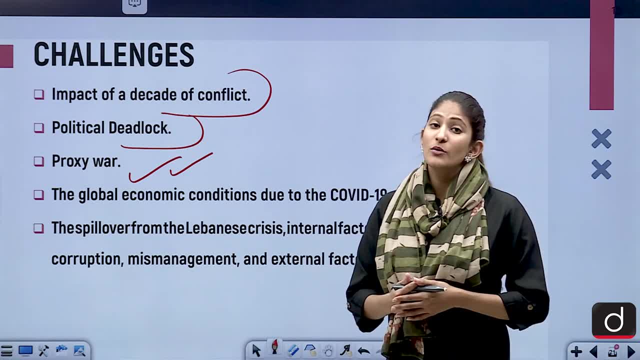 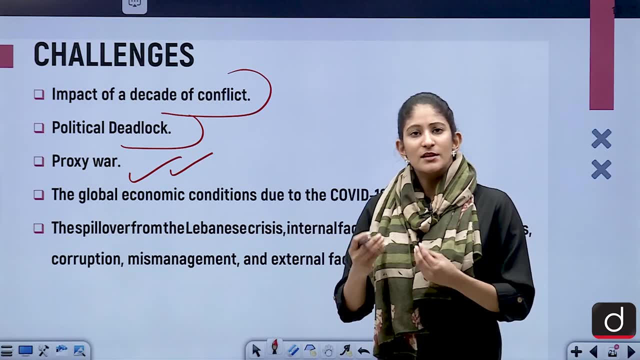 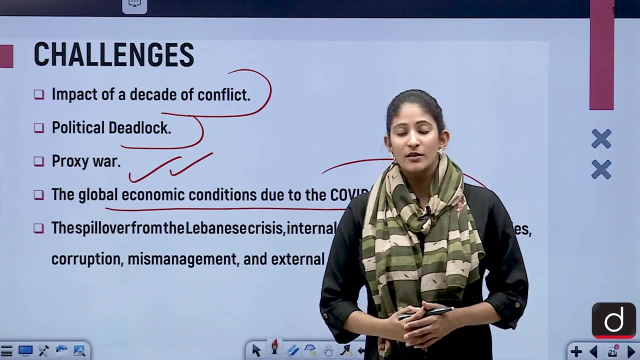 show their power. So how to control the proxy wars, How to make this country, the country of Syria, to have its own reformation, its own homegrown reformation? The global economic conditions due to the COVID-19 pandemic: not even US economy could. 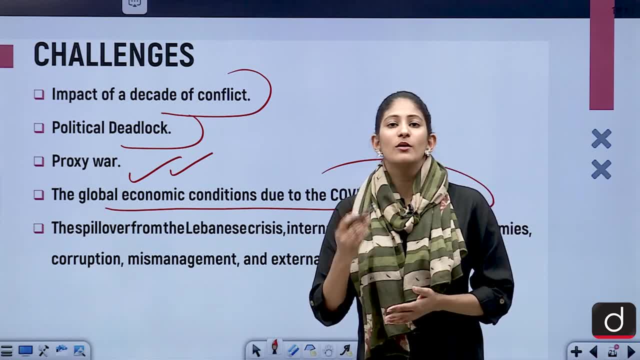 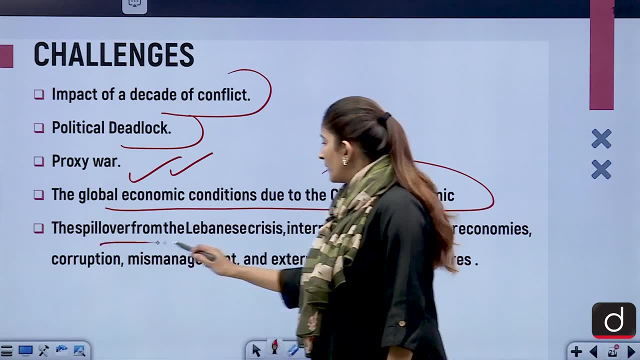 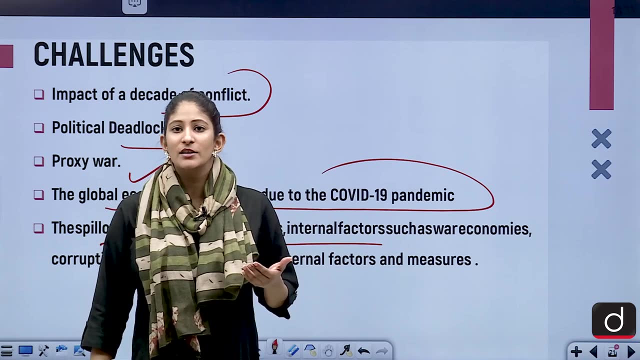 handle that? Not only Chinese economy could handle that. What about the Syrian economy? How we will deal with that? That is another problem: The spillover from the Lebanese crisis. There has been a crisis going in Lebanon which was aggravated after the Beirut explosion. 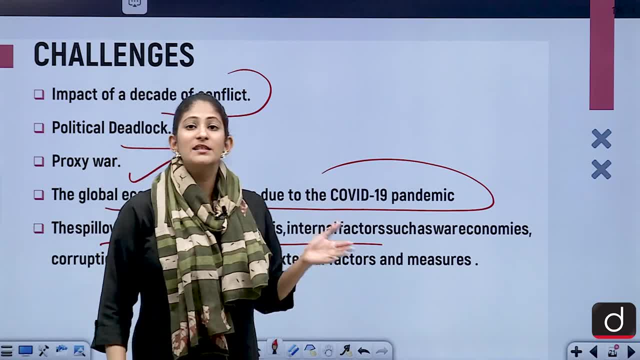 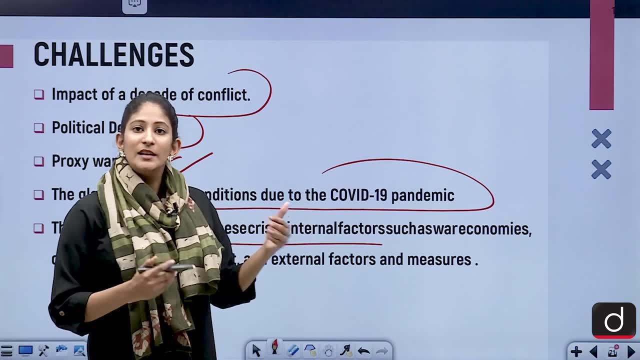 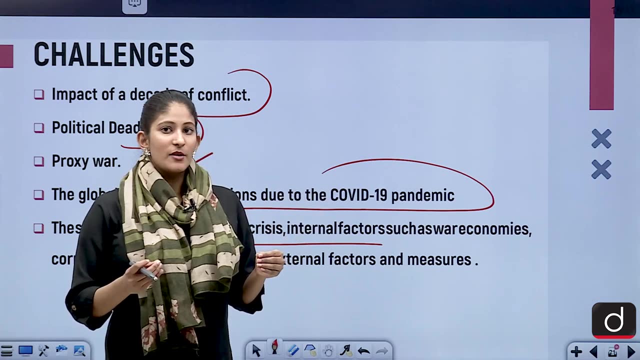 So after Beirut explosion, the Lebanese people started asking for help from France. The problem is as there, The Lebanese economy, because of being under a very, a very different type of government- That means an undemocratic government- it has been into the hold of that. 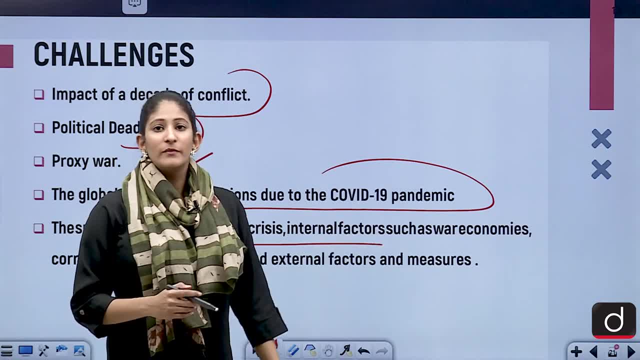 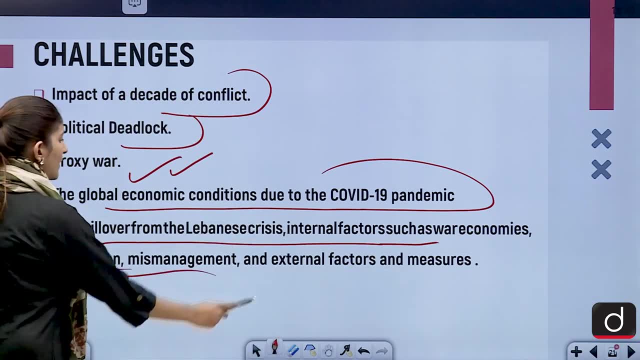 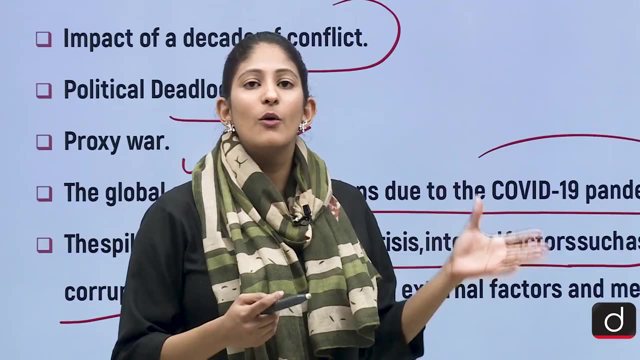 That is why the Lebanese crisis is also spilling over there. Right And internal factors, such as war economies, then corruption, mismanagement, external factors and other measures as well. So there is a problem, So there is a whole lot of challenge that the new, that the constitutional committee 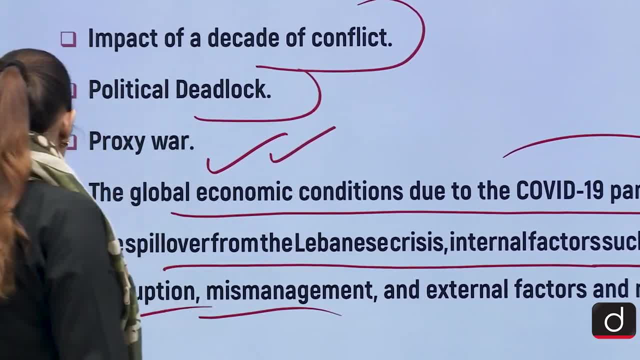 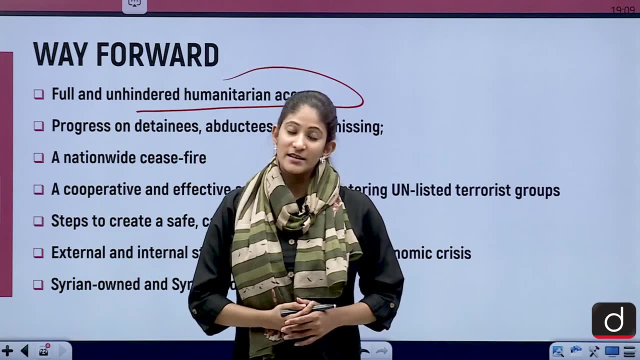 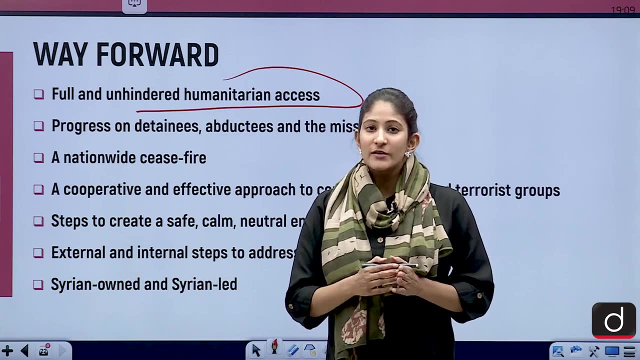 needs to take care of If we move on. So if we talk about the way forward, first way forward is full and unhindered humanitarian access. because of the war torn or war infested status of Syria, The humanitarian rights are in tatters. 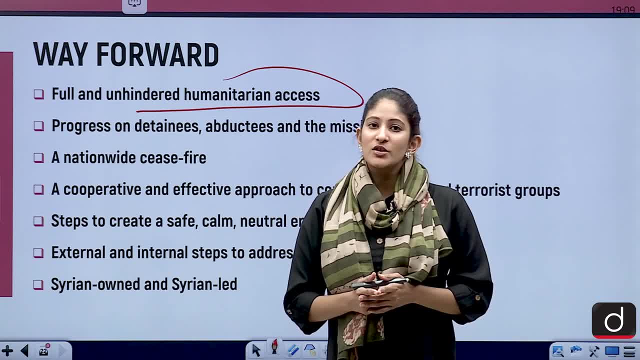 So to take care of that, all the countries under the aegis of UN should take care of them. So let us talk about that first. So the first way forward is full and unhindered humanitarian access because of the war torn or war infested status of Syria. 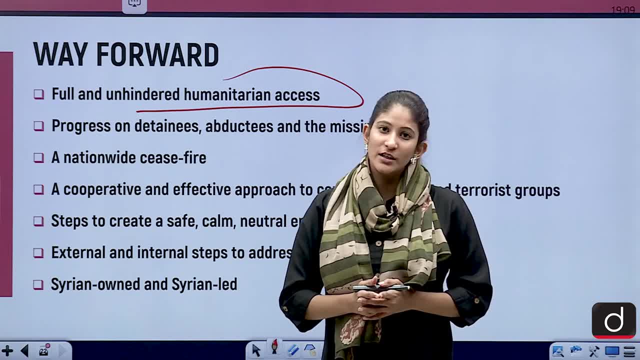 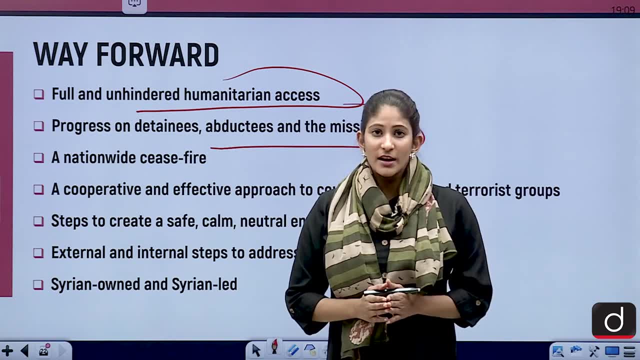 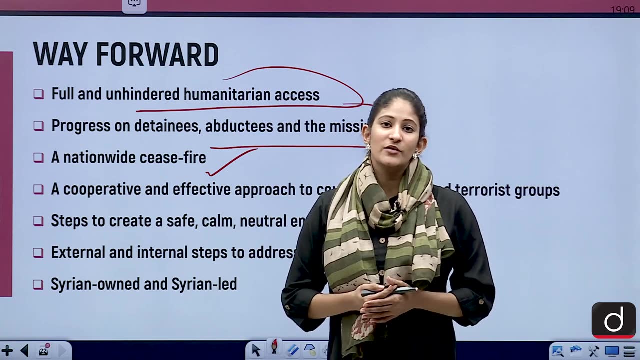 UN should be able to provide humanitarian help to the citizens of Syria. Also, progress on detainees. abductees should be checked in order to take care of the human rights, and also a nationwide ceasefire should be agreed upon between different ethnic groups, different religious groups, so that this 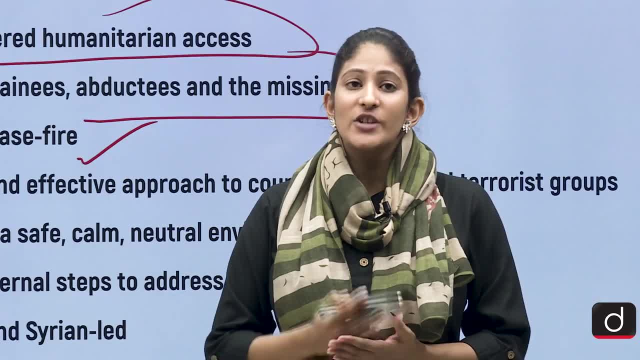 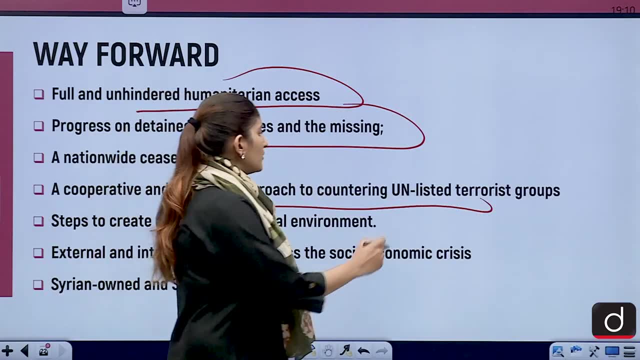 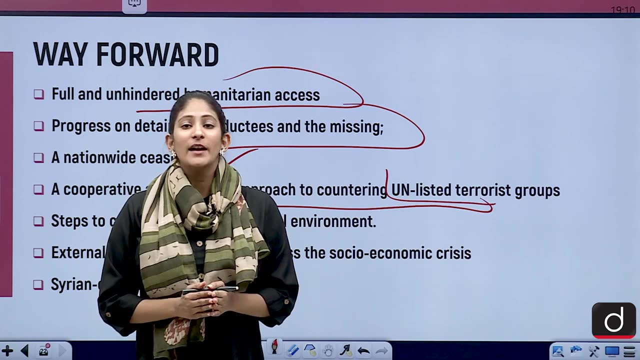 entire procedure of constitution making should not have bloodshed in it. Also, a cooperative and effective approach should be conducted in order to counter UN listed terrorist groups. There are certain groups which have been listed as terrorists by the United Nations. So a proper approach. 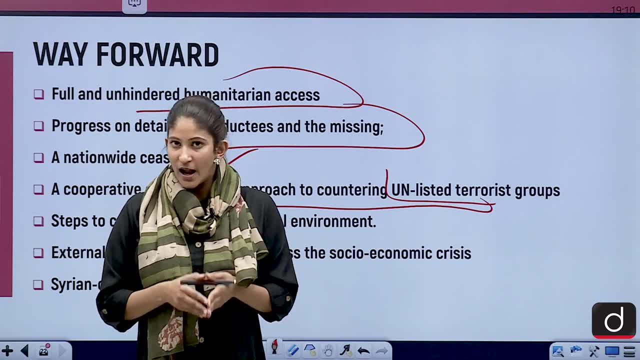 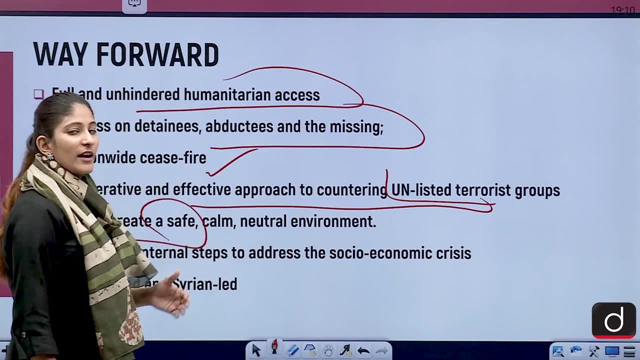 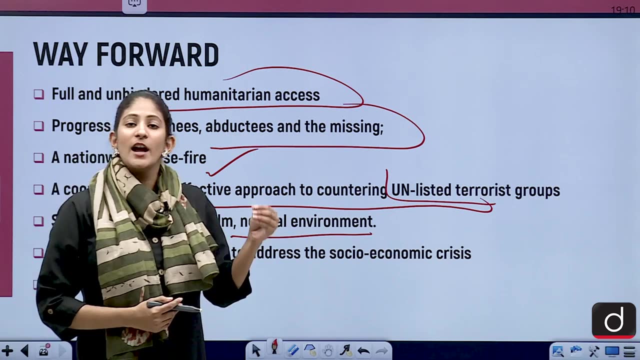 a coordinated approach should be led by the countries which actually hold stakes over the stability of Syria, and steps should also be created to ensure safe, calm and sustainable neutral environment Which can be taken care of, which can be sustained for a prolonged period of time, And external and 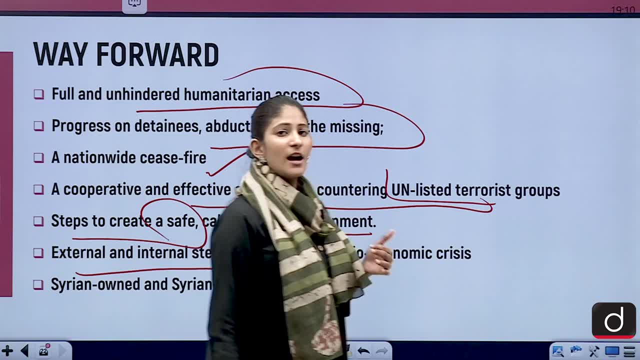 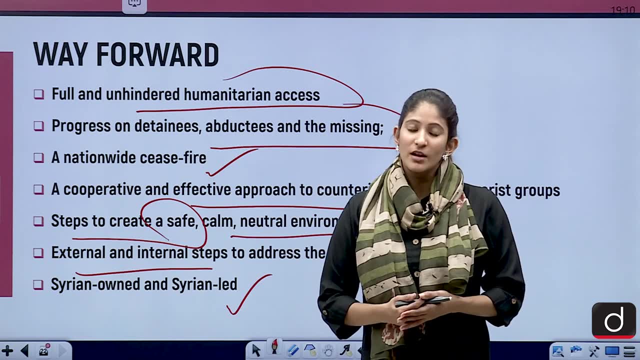 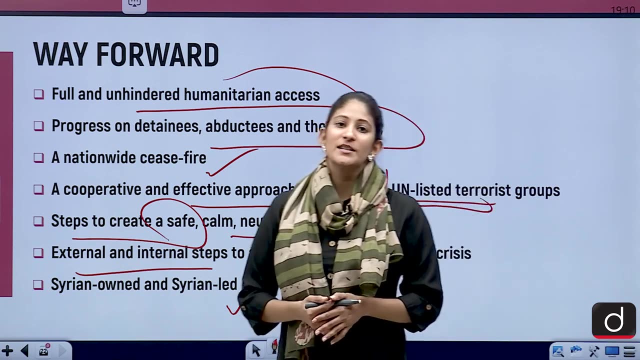 internal steps to address all the socio-economic crisis, especially after the COVID-19 effects and Syria-owned, Syria-led approach. This approach should be homegrown and not imposed upon by any foreign power. So that's it for today. Tomorrow we shall meet again with another segment. 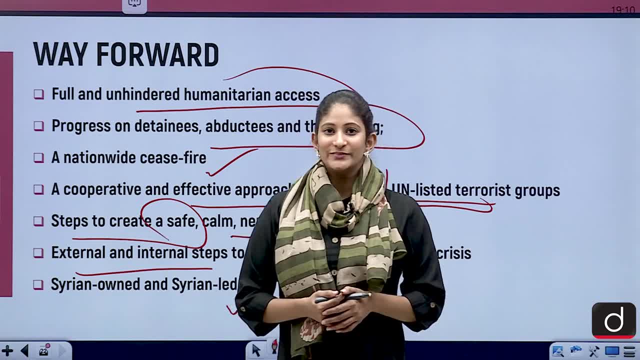 Until then, stay updated and thank you so much for watching Subtitles by the Amaraorg community.